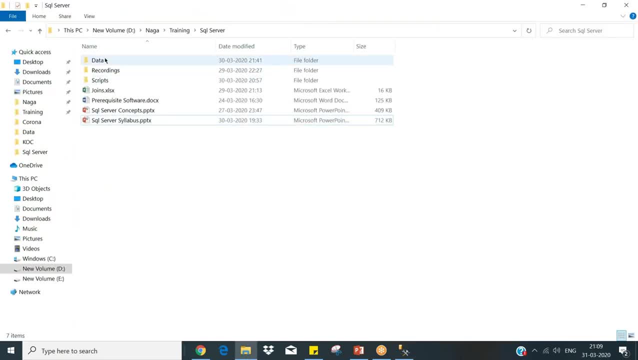 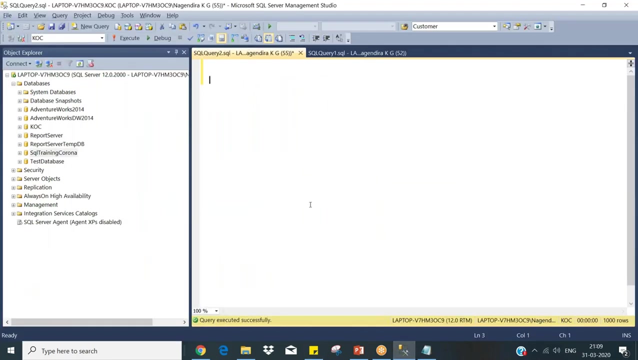 rate of multiple tables, you will always a query. it I mean yesterday query I'm trying to take. let's take this joints example: okay, okay, so this is the table we have taken today, so this contains a joint. okay, so when you want to have a join multiple tables, okay, we need to use left join in the gen, whatever. 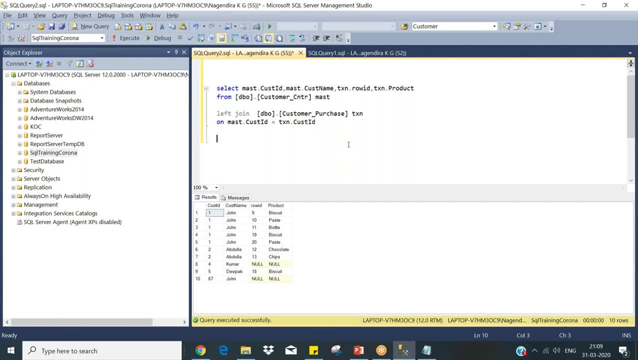 can be. so right here I will ask one question. so if we have a one table, do we not no need to create a view? I come again. I mean you said like if we want to join multiple tables, then you need to create a view. so what about if I have only one table? even with that, I can create a view, or not? 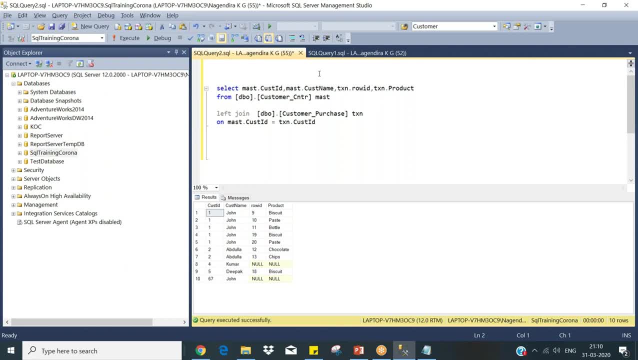 yeah, you can create a view with one table also, yeah, so basically it doesn't matter you how many tables you want to have. basically you want to store this query in the database object. that is the main purpose. so a view definition says: like it's on virtual table. now you can see like this is the result. 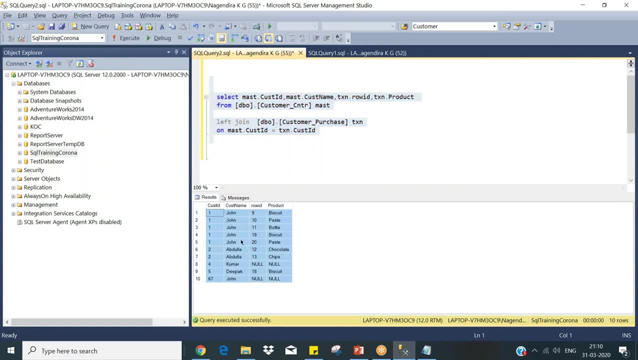 when you execute this query, whatever you see here. so this result is not stored, whereas this query can be stored somewhere in database. so that is the purpose of creating a blue create view. view name. your name is like customer, product purchase. okay, now you can start the database. 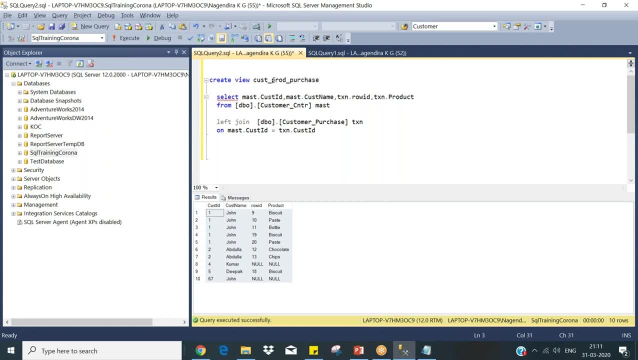 okay, so you always end up with having this kind of queries frequently. okay, you need to join multiple tables, and if you forgot this query somewhere, then it becomes very complex. so what you need to do is, whatever query result you want to have, you write that query and put it in a view. 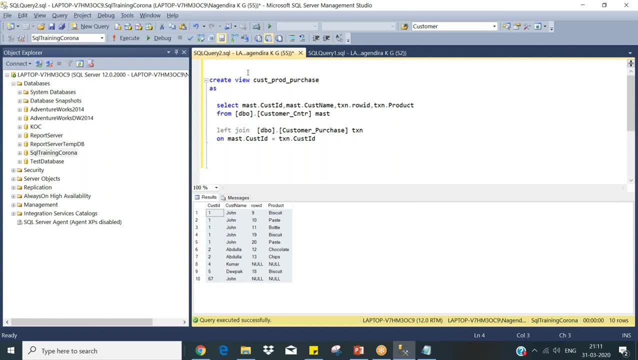 so this will create a virtual table. let me show it to you guys. so when you select this query, you are getting these four columns and with 10 rows. so when you create a view with this query, what it will do is, instead of selecting this particular statement, i can select this particular view. 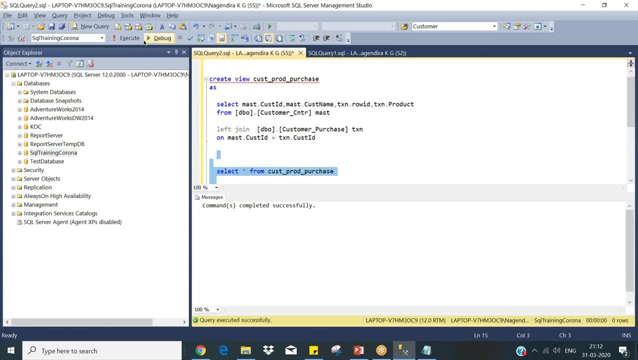 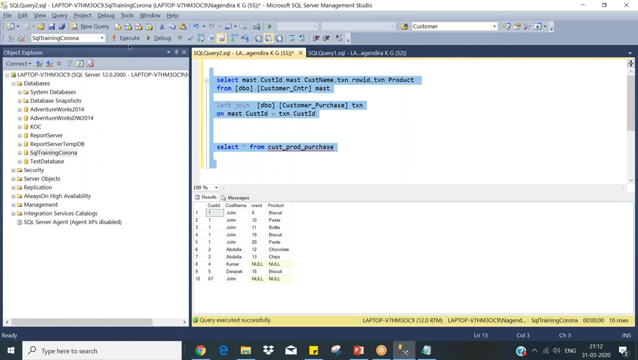 select from this one. okay, so you see the difference. even you can select this query if i remove this one, so this particular view is stored. now, you see, here you have the same result, even if you select the view or the query. okay, so basically you could be. 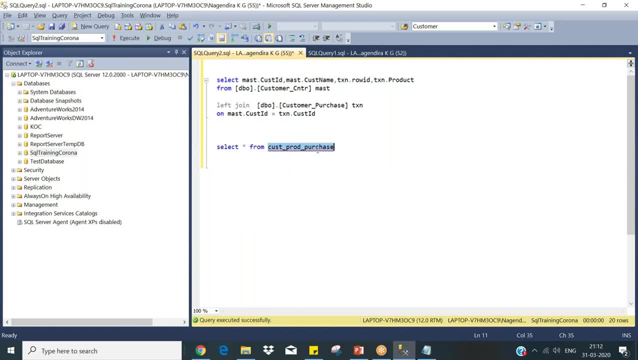 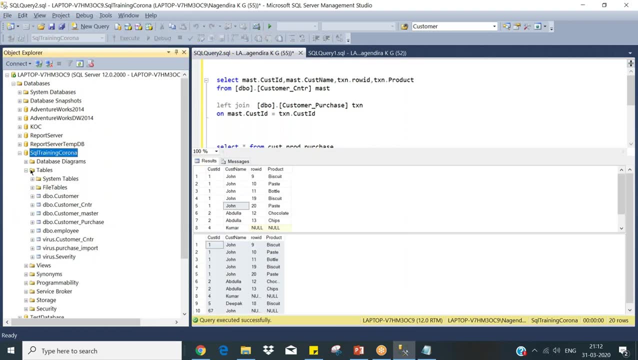 be stored in the view, okay, and the results won't be stored. so view won't store the data, it will store only the query. that is the main purpose of view. let me show it to you guys. so here it is the query i mean. the view is stored here: customer product purchase. so as 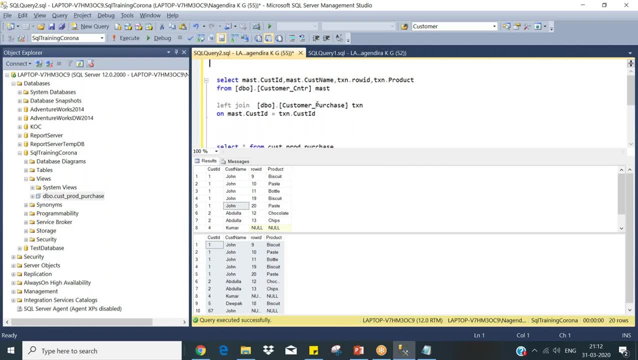 rachel pointed out, in order to have multiple joints, okay, so people will forget, or they use different joints sometimes once you use left joiner in engine. so this query will be stored. and if you use only one table, okay, and you use some var conditions where gender equal to male. 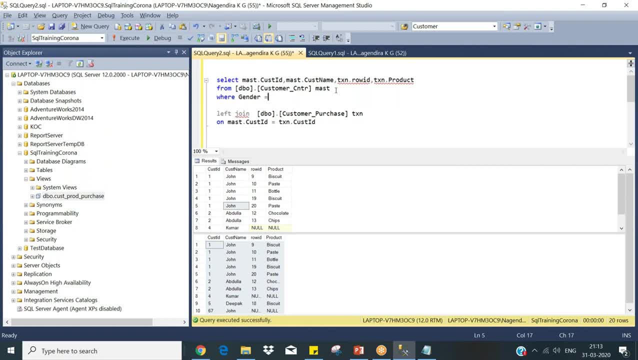 are kind of: i want to have some constraints to be defined. someone has some question: commonly used queries, uh, where we every time we will run again on a daily basis or sometime. so those queries, if we can save it, it will be easy to retrieve. yeah, yeah, so there are multiple. 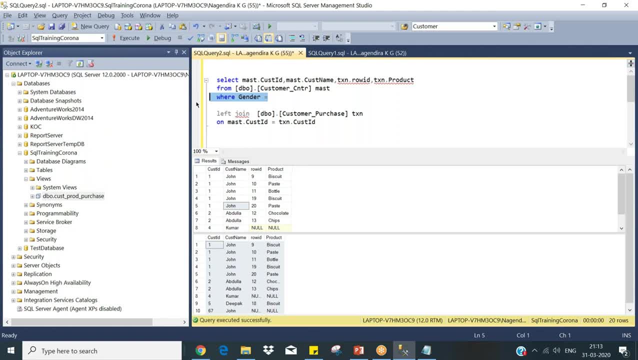 purpose. so it is not uh, you cannot store those queries. whatever you regularly use uh for that. even this is used for a security purpose as well. the views, um, the thing is like, instead of giving access to the table, you cannot, i mean, you can give access to the views. okay, so, as we discussed yesterday, giving uh object level. 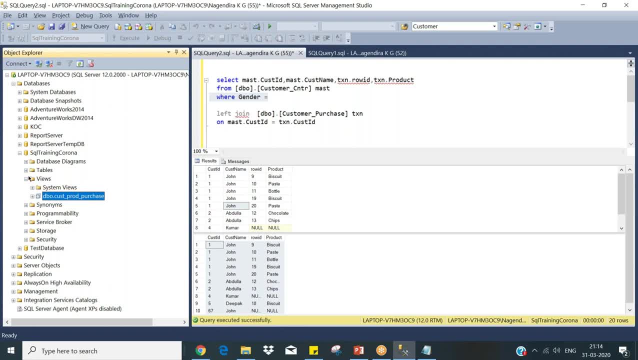 security. only the what objects you need to. only three tables are given for hr manager role or someone has a different username so you can give access to the views so he cannot able to do any operations in the view. only the deletion insertion can happen in the table. two is just a query. 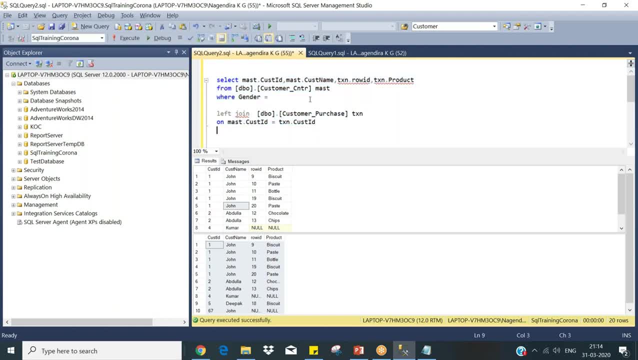 so that is main purpose of it. it is not only the common, that is also one of the purpose. but you say like you use a hundred to uh. i mean 10 to 15 quotes. usually you cannot store it as a view. just that query will be: uh, having uh written some useful information, always like this: 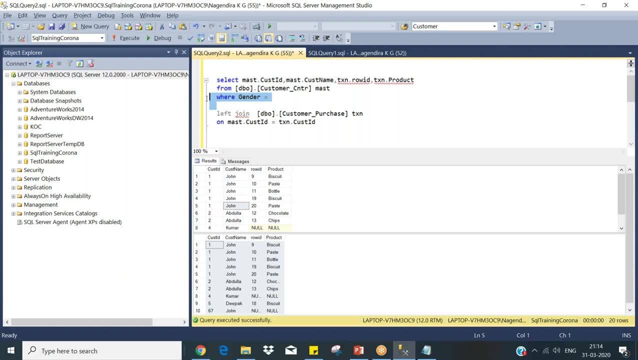 so i want customer product information. then you store it, okay, and that is main purpose. then you have something like um, security, security purpose. instead of providing a table access, you give access to the view. that is a two- uh, important purpose of creating a view. so, in the view, what you can do, whether you can do a delete or insert. 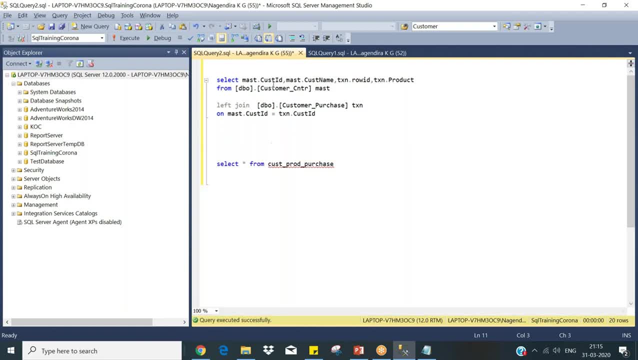 as i said earlier, it will create only the virtual table. you can have only the varkandi- i mean select statement inside the view. so what about? uh, order by class. create view customer purchase. this is customer purchase. i have a customer purchase select staff from. even you can create like this. so this is used for the varkandi. 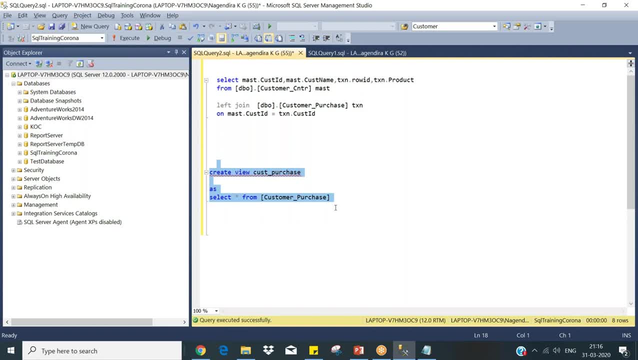 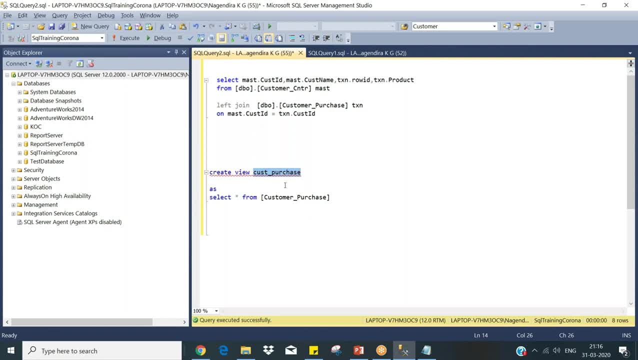 name. instead, you want to give your access to customer purchase. so you are. this is used to hide the base table information. there is multiple purpose for creating a view. so when i create a view like this, only with this stable information: select starvon based on the table information. select staff from. based on the base table information. there are multiple purposes for creating a view. so when i create a view like this only with this table information, select the28 knitter it is couple on Из or alt key��. last name and lighting download is 이것 21 Direną thousand bricky gear. return to. 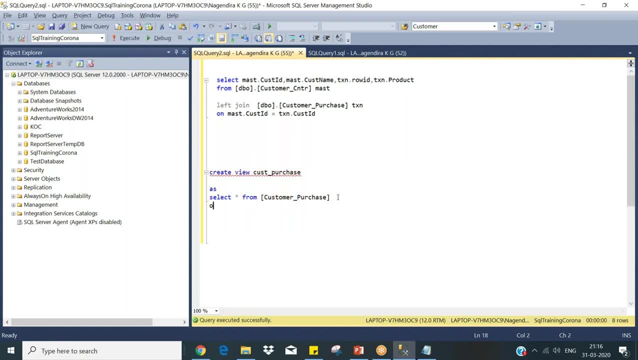 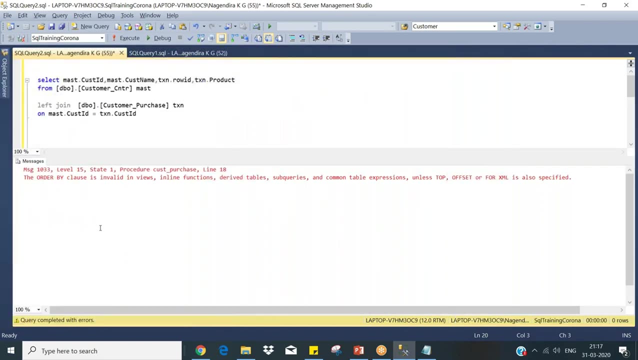 are from, based on order. i think it should not allow order by row id. i don't think it will create. see, this is another important thing: you cannot specify order by class inside the views- inline function, derivative table sub queries, all those things, common table expressions, all other stuff, because it will store only the result, whatever order it is fetching you. 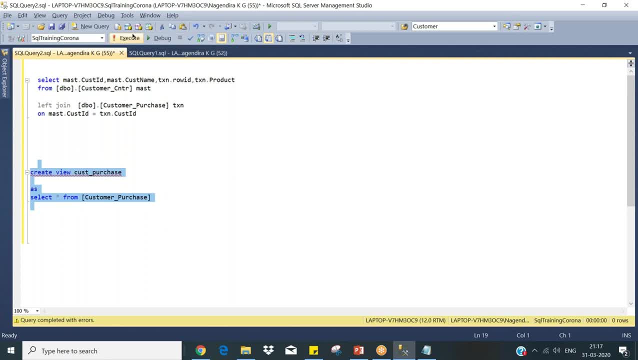 cannot specify it here, but once you create the view, okay, then you can specify the order select. i will comment it out so that you can understand: select start from i'm selecting from the view. okay, then order by pro id. this is simple. i mean, it is as usual. you can specify the order by: okay. 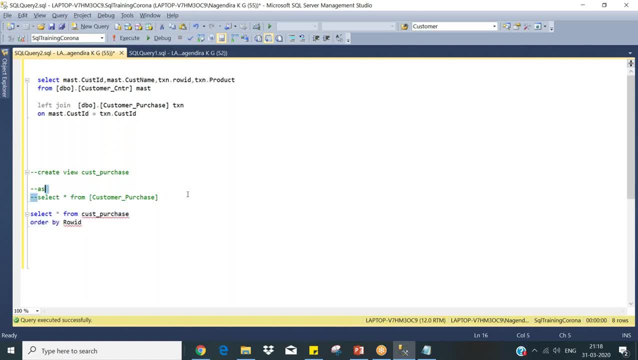 because it it is storing only the structure. okay, it will not store what order you need to store. so that is what it is restricting. these are certain limits and limitations and using a view, but it doesn't make any difference for you guys. okay, with this note, let us focus on another topic: common table expression. 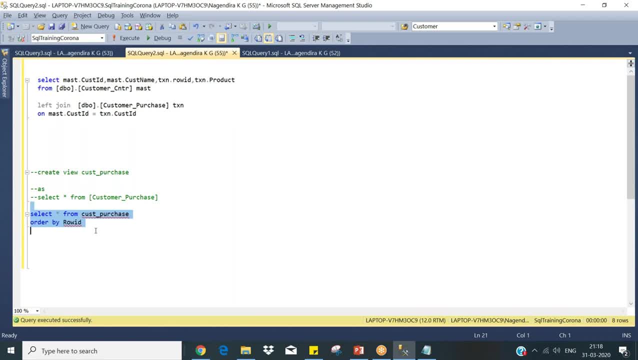 so i have said like: uh, we have created a view here, okay, and what about? uh, i need some results to be stored temporarily. so i have created a view here, okay, and what about? i need some results to be stored temporarily. so i have created a view here, okay, and what about? i need some results to be stored temporarily. 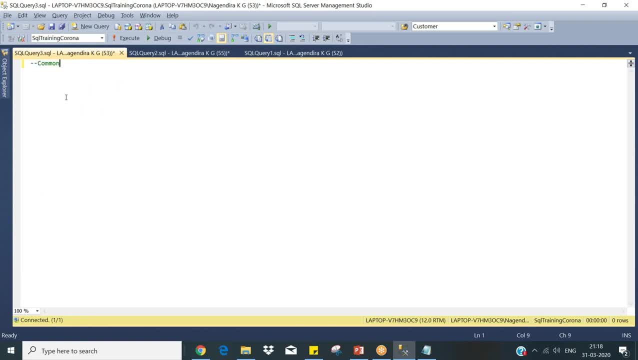 so i have created a view here, okay, and what about? i need some results to be stored temporarily. for that, we have a concept called common table expression. okay, let us have one example here. so you have a customer, john, and biscuit, everything. okay, i can, i want to, so i want to filter out. 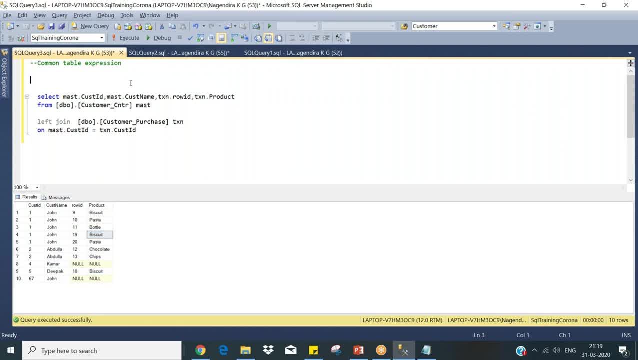 whoever bought biscuits. okay, so what i will do, i want to use some biscuit and, uh, chocolate, these two conditions, so these two things. i will try to get it in another table. i want to put it in in condition here, in condition, into the yard, which is what kind of the table i want to put in the week in condition here. i want to use in condition, on which unit in this case? let's check it out here- i want to use in condition my writing area, just to make sure it works. okay, then, for the пишive, with a few steps here, two methods. so i have two things. so i will give you just a few things, but only for one, the table. so i want to use this one, a few steps, but only two steps. i want to input of the other table, which is code and very good and again because all the field, so that you can varying the what. 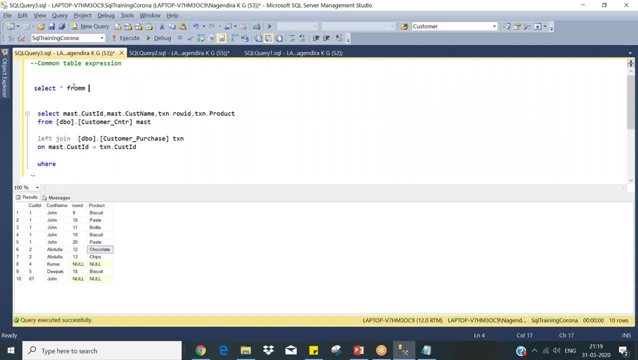 So let's start from. I can do like this as you, you. you need to create some template table and those results. you need to filter it over here. Okay, Our product in with them. product Yes, Okay, So this is a way to create some temporary results. Okay, Select star from see. see here. 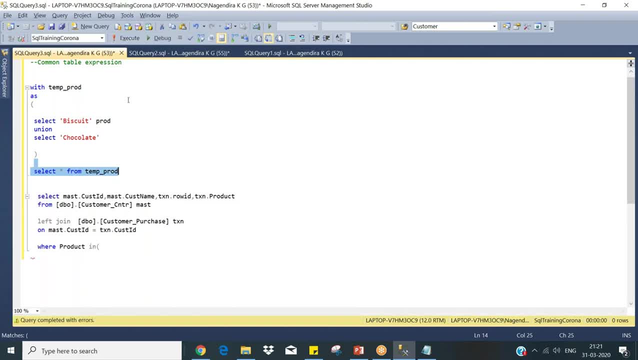 If I select this statement, it will throw me error because, whereas when you create a view, after creation of the view, this is an object created in the database. I can able to go and select it Okay, Without choosing. that one creation is like your object is created. 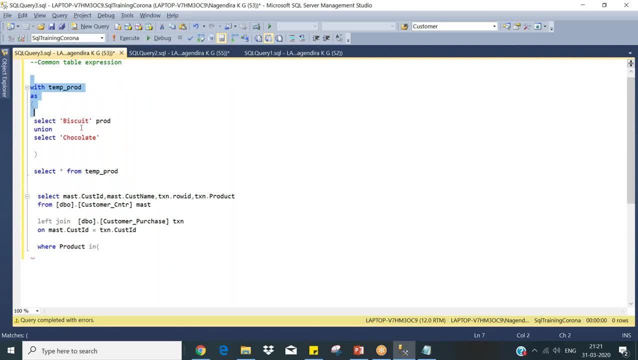 The metadata is created, but it's a common table expression. I have this one here. Okay, Even I do like this. Okay, It will throw error because it should have the width statement should follow with the select statement to see here. Okay. 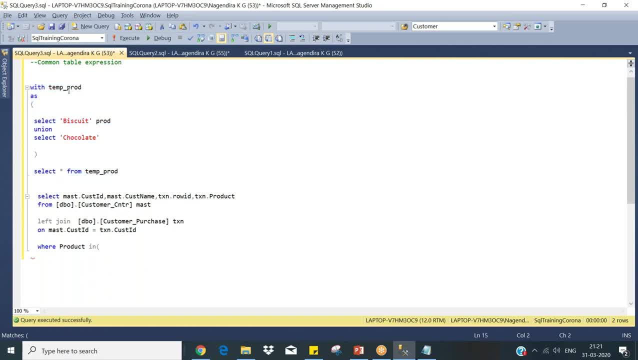 I need to select both with and select statement. The width should followed by a. I mean the select statement. Okay, So this is the thing. like I have created some temporary results, I want to store it. So this is nothing but your common table expression, which will hold. 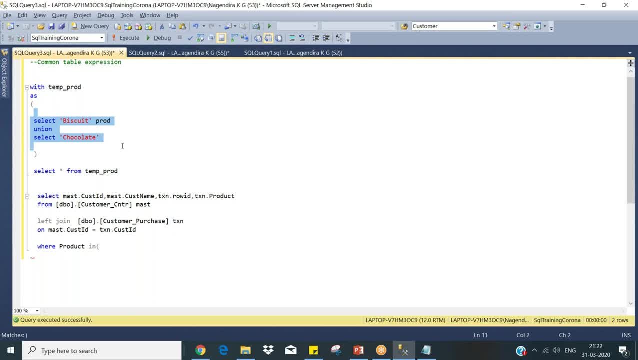 some temporary results. This can have any table information. Okay, For simplicity, I have created two rows and which is having only one table. Okay, So this is the thing. I have created two rows and which is having only one column product. Okay, So this result. 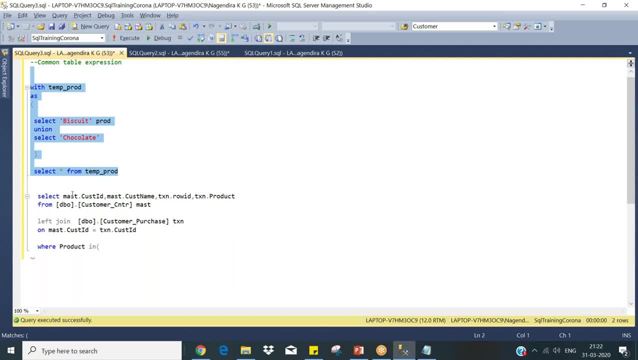 what I'm going to do. this should be acting as a filters. in this particular table I want biscuit and chocolates. So select product in. you guys know about temporary tables, I mean sub queries. select broad from: Okay, Okay. 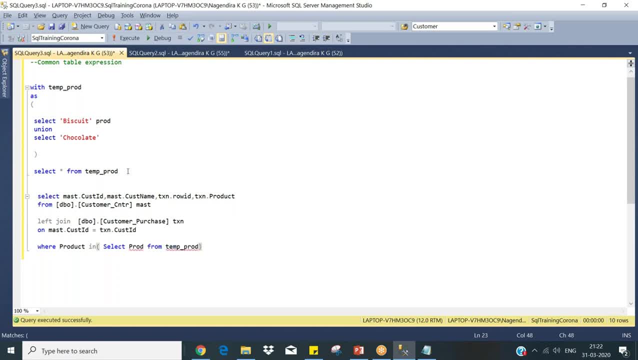 Okay, Okay, Okay, Okay. Yeah, Let's see. First I'm going to start with this table, So once I select this, I need to comment it. As I said, this scope of this table, This comment table expression, is within the next select statement, So I should not use. 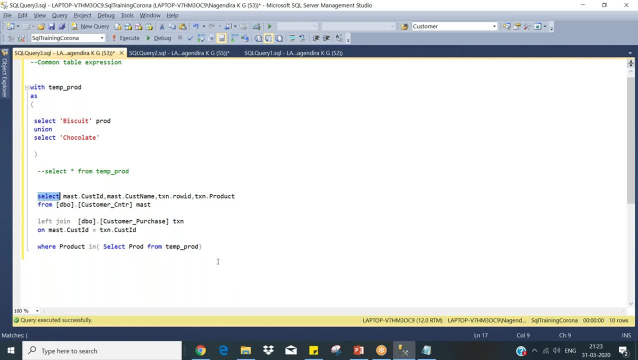 this I like statement. I need to use the select straight. I got or purchased biscuits and chocolates. Okay, Yeah, Yeah, okay, this, this column, i mean this, you can mention it here also. okay, biscuits and chocolates, something like that. but assume you have, uh, you don't know how many. 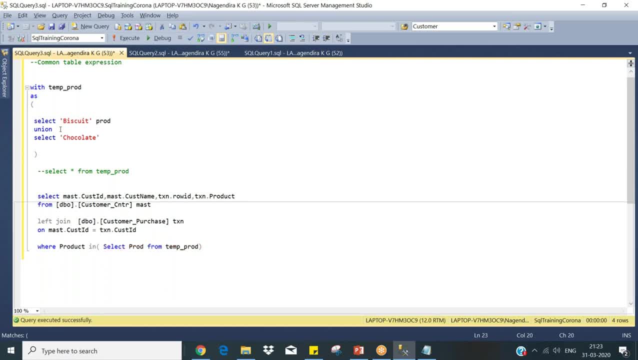 records it's going to fetch. whatever query it's going to fetch here. you remember some queries like whoever has this degree and the employees whoever has this designation. those employees should be filtered, something like that. so in those cases, if we don't predict the account have a discrete values, the result set will be based on the conditions over here. 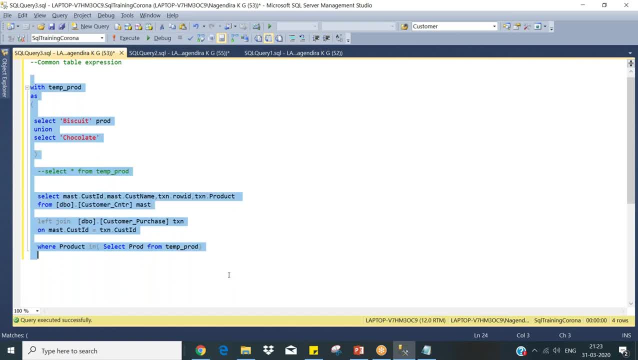 in those cases you can use such a common table expression. okay, so a view and common table expression is different. this will exist only with this query if i use the same table reference after the select statement. if i run along after the select statement, this will not execute. invalid object name: temp broad. 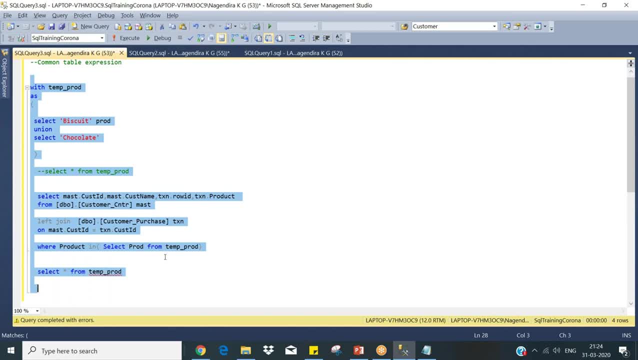 okay, so that is the scope scope. you understand, i think, the scope statement, scope of any statement, how long it will exist, whether it's a global or it will last for the session, all those things. someone has a question. this union is uh, will combine both the select statement, right? 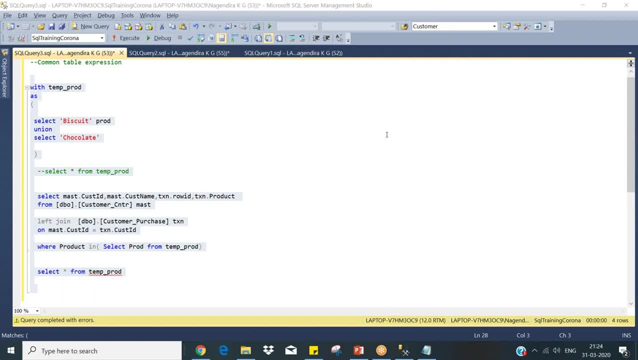 data uh union. you have included select biscuit prod union. so this union will combine both the data. yes, yes, yes, get the data. yes, yes, yes, it will uh append the rows. amend the rows. this is row one, this row two. maybe you for confusion, i'll put it as id. 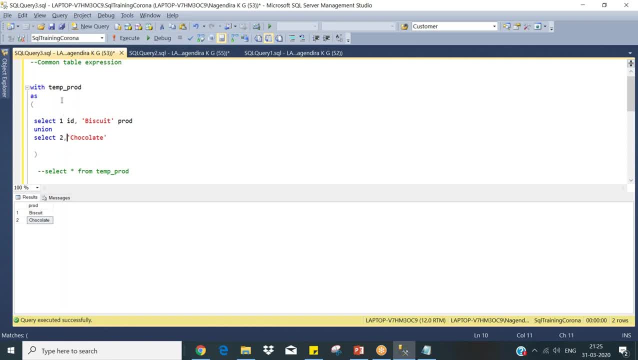 yesterday, i think, union and all i taken last session. if you will do that, then this is going to the table reserved, the. this is a width. okay, the view definition. you just try to um compare it with a view and a common table expression. view is permanently stored in the database. that is common table expression. 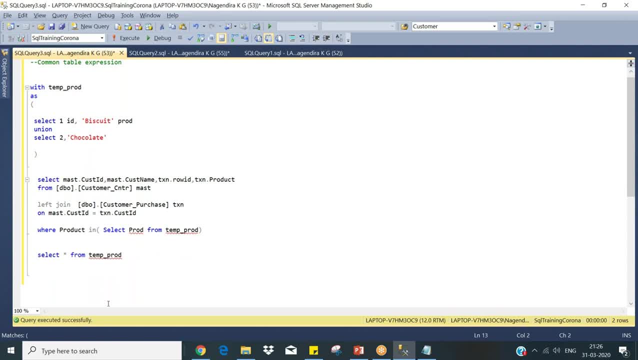 the scope is within the next select statement. even if you use here, this won't work, but whereas if it is a view, you can create it as a view. if i change this one as a view now you have seen like this: result. you got result for this query. you got error for this. 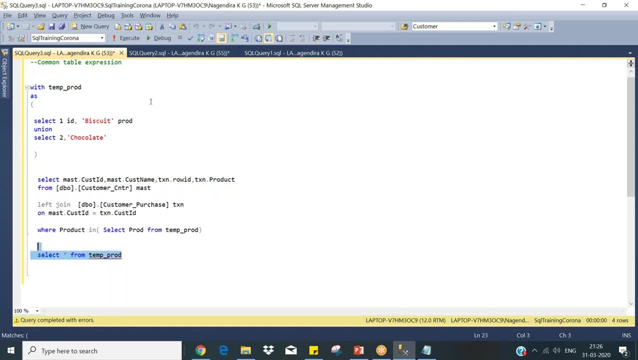 select statement error over here. okay, what happens if i create it as a view? create view. okay, even you can do like this view. first you need to create. you cannot take you along with this. just execute with that. two select statements. now you got the output. okay, this is the main purpose. when to use, when not to use? okay, now there is something like: 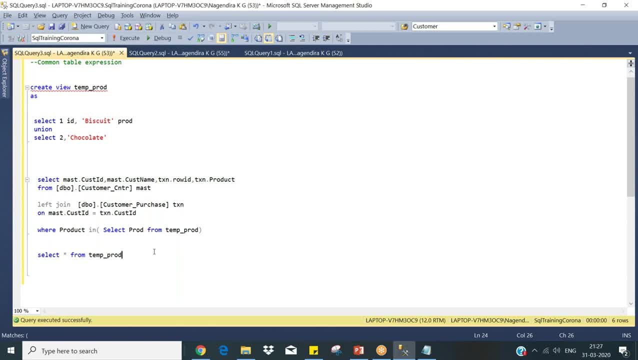 common table expression similar to that, you have, um, something like temp tables, temp tables. okay, there are uh, two types, i think. for now, i think you can stick to two. uh, hash table, hashes table. hash table is nothing but local tim table and hash test table is nothing but a global temp table. 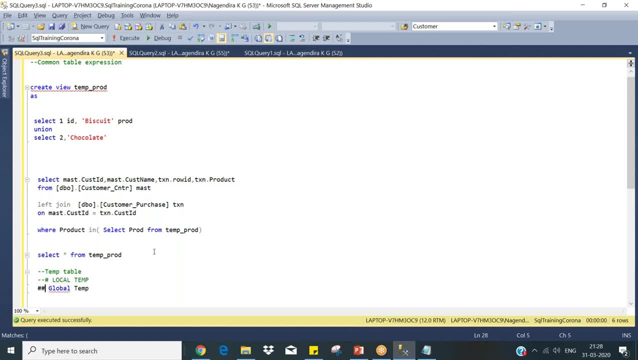 global temp table. maybe you have two types available. yeah, okay, okay, good, so, as youYawn, manager, if you are still watching, mainly audience guys, so what is those? so all these things is the temp table purpose is to store your results temporarily and when, well, the purpose of the table is met, then you can drop the tables. that is the main purpose. 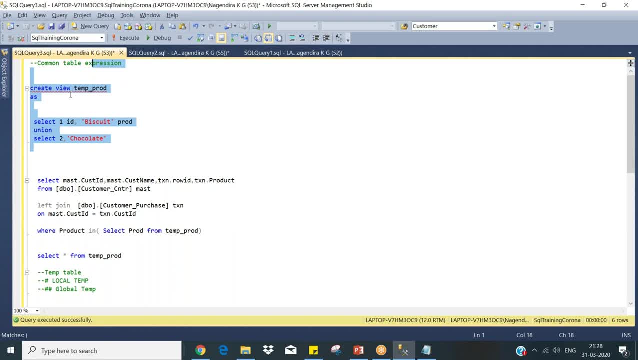 this can be stored in a view. this can be stored in CTE. now I'm going to store this result in temp table. so say, for example: it is like create table, the temper table is same as your normal table creation, but you need to prefix with the hash ID and you say product integer, say care of 20. 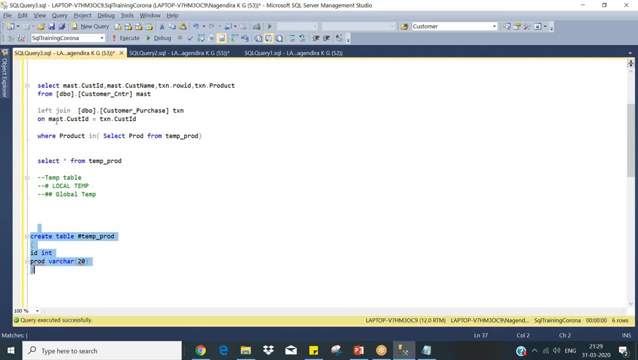 okay, I can. I am going to create another table and say global temp product and prefix with hash hash you. so this is the one. now. let us insert these two records temporary table insert into. okay, it is as simple as that. let us insert for global table as well. 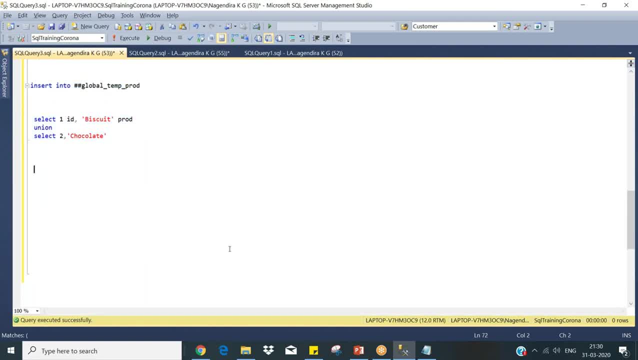 okay, you, you, Mi. so what is the difference? why? when to use, when you should not use global, when to use local? those things I will explain shortly. we both have data. okay, here now I will take the type data available for potential Neurilheal start. okay now, once I, Uh and I have prepared the total data, okay, so we will start using global. 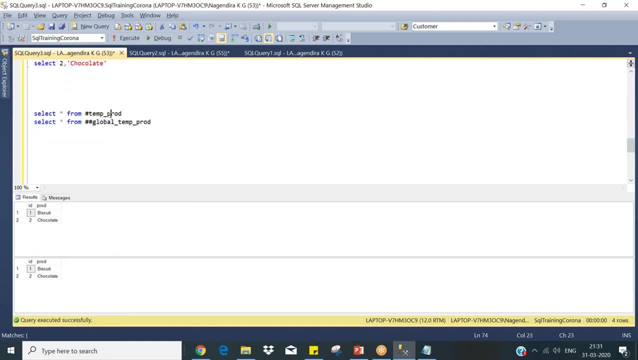 Ready? now take the total tab in case you don't understand why, if you don't have ум sentence, but you don't, this guy, this local temporary table and put it in a new session. let us see. whatever you create a new query here? okay, that will have a id, if you can see at right end bottom when. 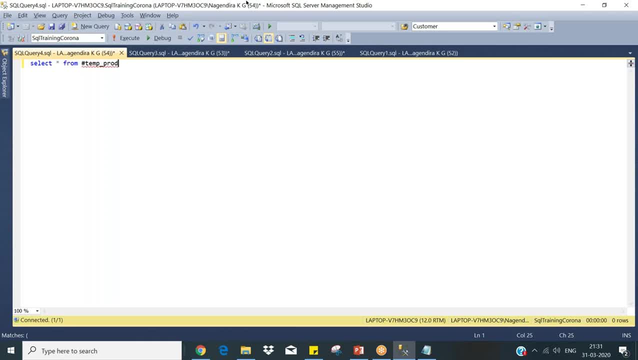 i highlight. there is a number after my name, 54, then over here it is 53. this is nothing but 53, 54 and all session ids. okay, so you have created this local temporary variable in session 53. you cannot go and access this temporary table in another session, but you. 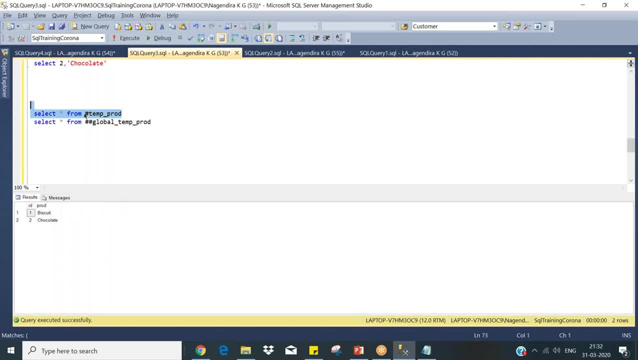 can access within the same session. so the scope of local temporary variable is within same session, whereas hashers table i created here in session 53 i can go and access in a new session. okay, so this temporary table and global temporary table once you drop wherever you are created. 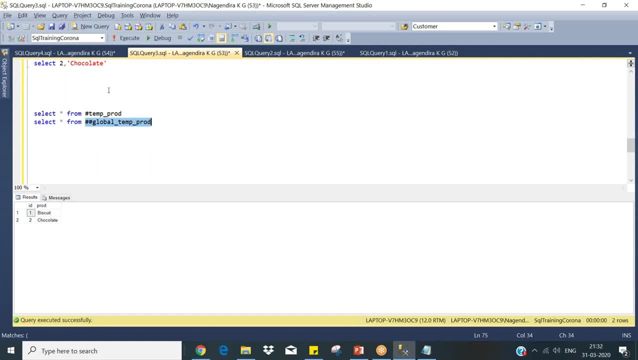 once you close this guy- okay this session- then these temporary tables will be dropped automatically. so i can drop it manually also. drop table like this, drop table. so the all other operations altering table, whatever operations you performed in the table, those operations you can do it in this table. the only purpose is to store. 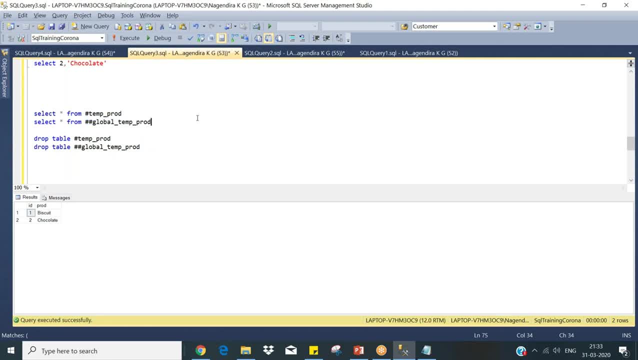 your results temporarily okay and sometimes so, where you will use okay. basically, let me answer this question. so basically you have a next. next i'm going to talk about the stored procedure, where you keep calling one procedure from another procedure and sometimes what happens? based on different applications, you, you call. 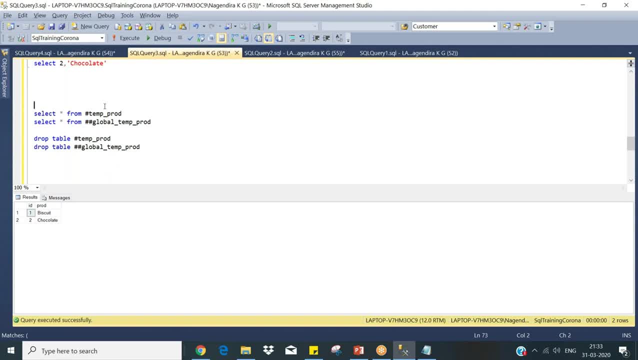 some data called in one session should be accessed in another session, okay, and in the in those cases, and that results should be stored temporarily. so in those cases you will use global and some cases like within the procedure or within the execution of that batch- okay, all these things. when i go and execute as a whole query, it is called batch running when i run. 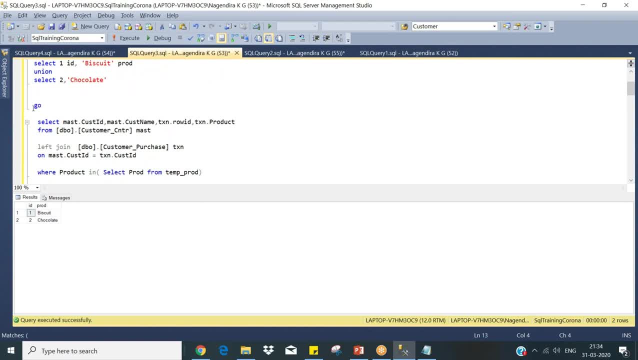 the batch starts from go. when you have a go statement from this go statement, whatever statements you execute, it is as a batch. okay, in procedures you use go statement, so within that go statement it's running as a batch. that will create one session, so your scope should exist. 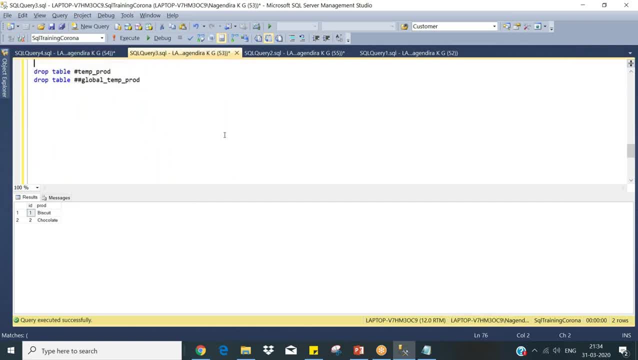 within that batch or session. then you use local variable and your data should reside for other sessions- i mean should be available for other sessions- then you need to use global temporary variable. mostly we will use this one because our logics is not so that complex. so this is good to know. and what is the purpose of common table expression that is used to store? 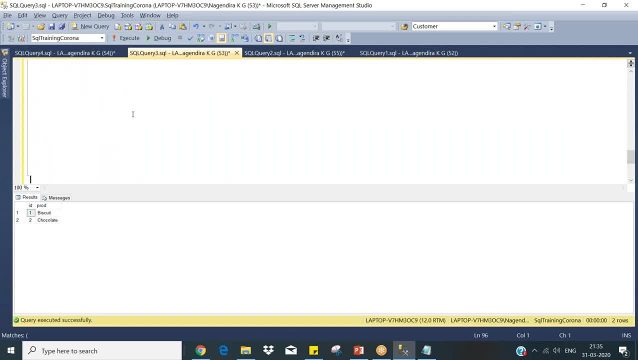 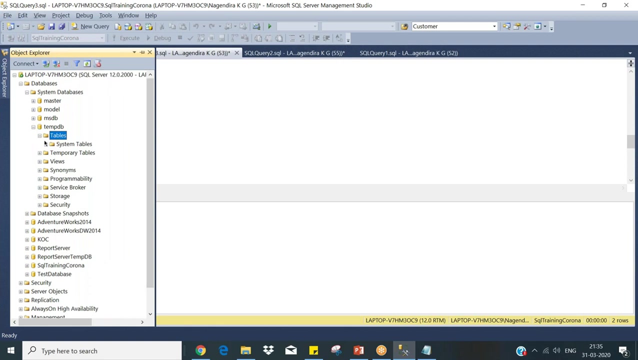 small results. basically, there is a memory logic behind all these three: local, global and this is your cte. okay, there are some memory requirements. this temporary product and temporary tables stored in your system databases, stem, dbs. i think it will have somewhere over here. temporary tables: see global temp prod. global temp prod. 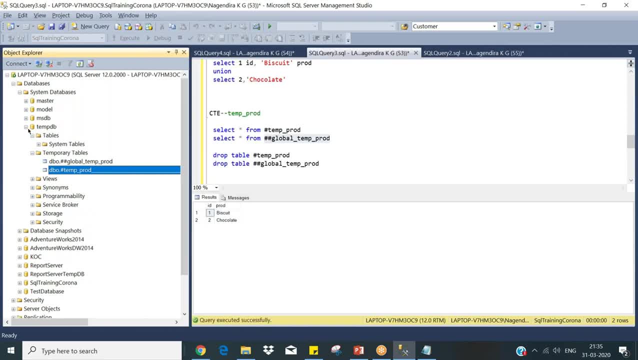 so it will be stored in your, as i mentioned earlier. what are the system database? you have a master model, msdb, temp db. so when you create a temp db here, it will create a temporary tables here. so physically physical table is created, okay, whereas in cte you don't create a physical table. 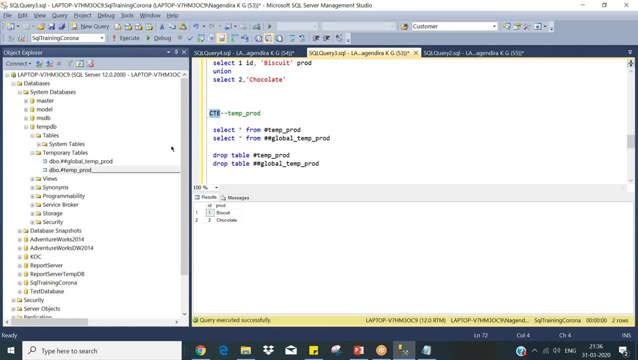 anywhere in the database. that is the main difference. so you might ask why i need to use temporary tables. instead i can start with a temporary table. instead. i can start with a temporary table. and here you can see that my 210 thing. there it says in cte: there five parts, there is a. 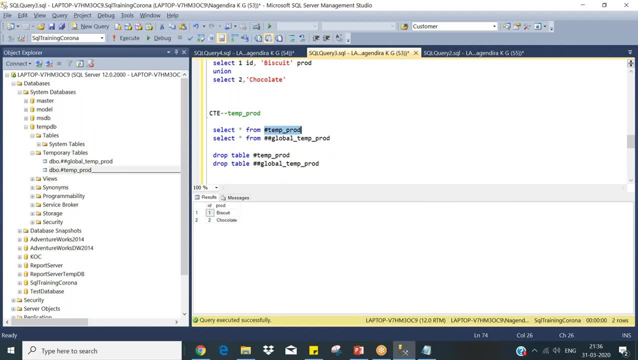 represent you, you can show the results and cte within the scope. so usually if the volume is huge that requires some storage, go for local temporary variable. otherwise if you run it and the cte, it will be stored in ram. so whichever isn't stored in the database physically, these things will be. 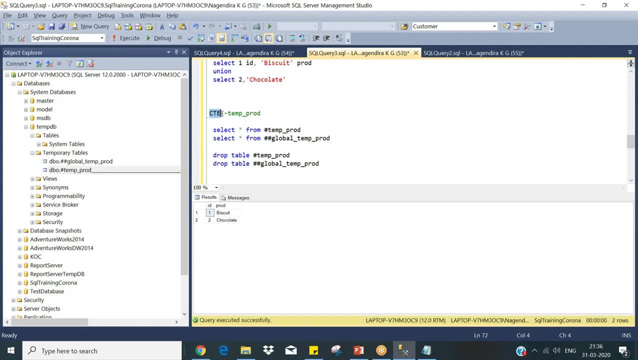 stored in ram, so better avoid it. your system performance will reduce. say, for example, if you're studio store, show for temporary tables. such cases you need to take a call based under okay. and if your temporary table should be accessed by different sessions, go for global temporary tables. 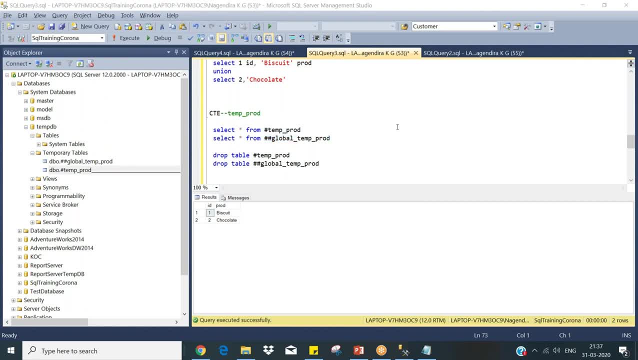 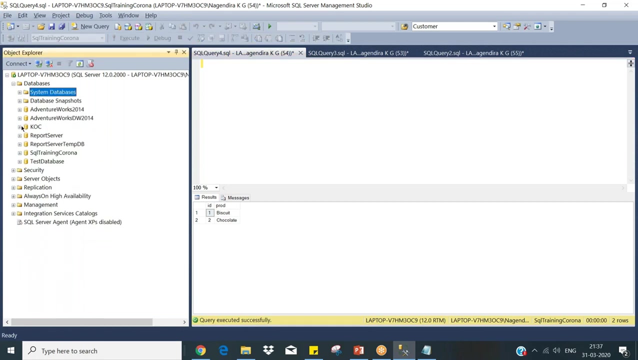 all right guys, any doubts in this? no, okay, fine, let me proceed to stored procedure. so we've seen about these tables, views, the purpose of views. you are all your predefined queries and used for this table. so let me proceed to store procedure, security purposes as well. now let's go little on programming part. 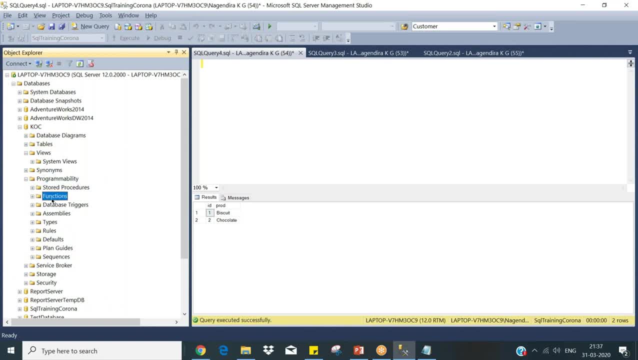 like stored procedures and functions, all those things. let's start with the stored procedure first. so, similarly, you have your queries written okay in the views. you have only select statement. what happens when i have some data querying or data manipulation language? i need to frequently update one particular record- customer information- okay, whenever i receive. 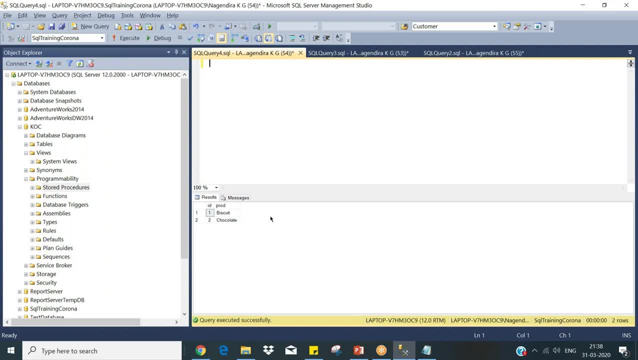 in the forms you have like. as we discussed earlier how the data will get into a database from business perspective, you have forms in front end. they create a customer, they press button, insert, or i mean submit. you will get insert into statement, into the table. so you, you can, you, you can submit claims or, if you will, a request for a. 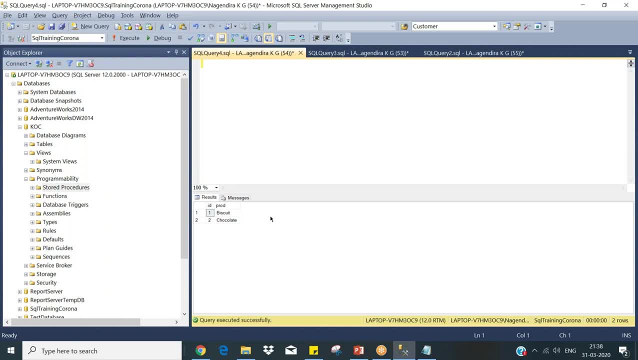 reforming event. you will have that part of the laid out by the library if you want to téléphone call, but of course that doesn't wait too for now. if you want to update your �aro constitutional change to this scale phone number, you will do it in the mirana application first time. helps, alright, and that at that once complete. so something like this kind of address most of time is: and now, because you have your unstable website or written code but there is apréski every time, then you'll have to update your Ouch correcting systems into localities- sometimes, likewise when i want to do change in my customer information. so what we need to do, we need to do the update correct, so update each time. you cannot run one code. i mean that stupid. i mean that piece of code is by default what you need to pass. usually people will update a phone number, people will update the donuyard, will update a number, yes or no. 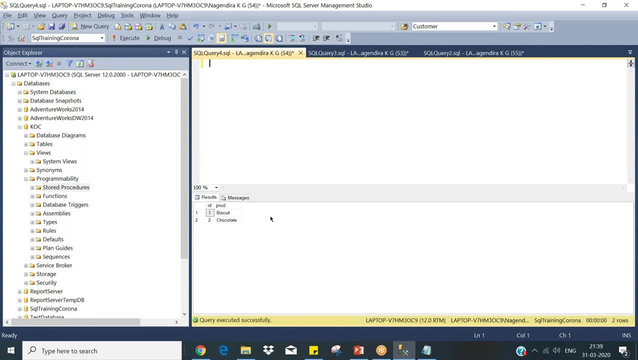 will update address. so what information you need to update phone number or address based on what you need to update customer ID. so this is a predefined structure and I'm going to repeat for n number of customers. if I write a code once basing, passing a parameters, then customer information will be updated. 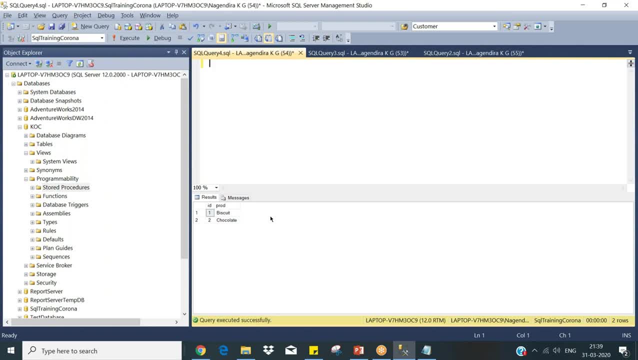 just passing a parameter. so these kind of scenarios: you create that code in a procedure. okay, that is what the one of the main purpose. you go for a procedure, repeated task. you want to do that code to be executed every time some operation happens. then you go for a procedure. let's have the same example now. I'm 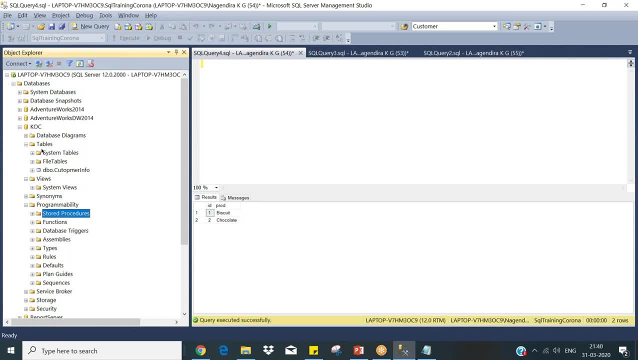 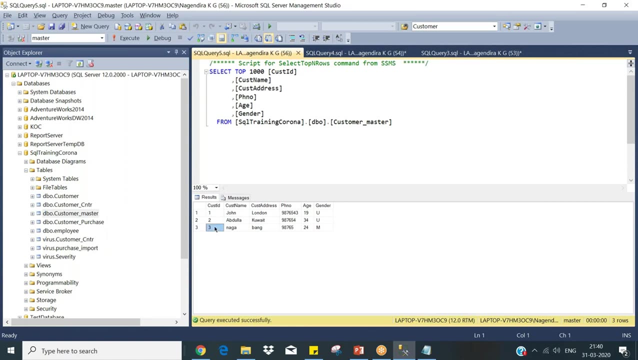 going to update information. SQL training: Corona, customer master. okay, here what I'm going to do. I give a customer ID. okay, I will pass customer address and phone number. okay. when I change any of this information, my information should get updated. okay, I will pass customer address and phone number. okay. when I change any of this information, my information should get updated. 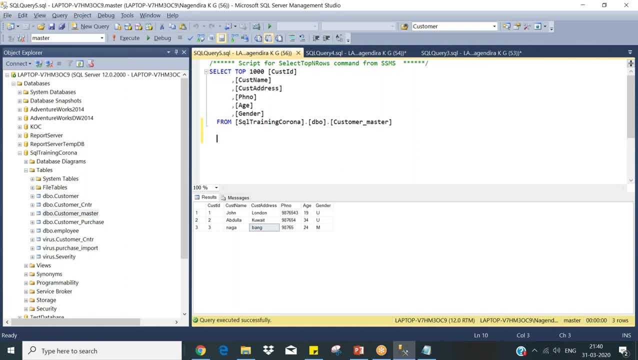 so how to update? usually we write update query right, update customer master, set customer address. for simplicity, I will go for a customer address update. for now, okay, and we can focus on another parameter later. customer address: I will say like I have bangalore and moved to Chennai where customer ID equal to. 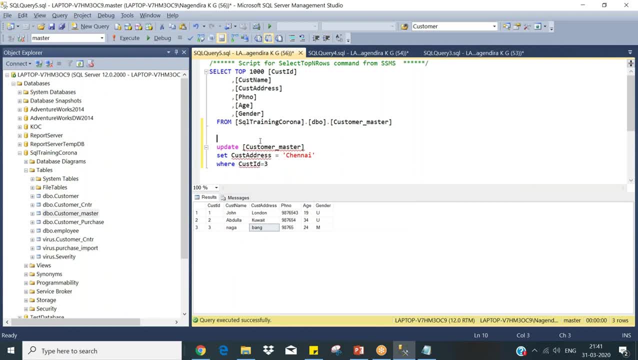 3. so what it does, it does like for Naga- you update the customer address to chennai. let us try that one. why i'm not in a correct database? okay, this is the thing. now you see the same information now from naga. it's moved to chennai. now you got it right. earlier it was. 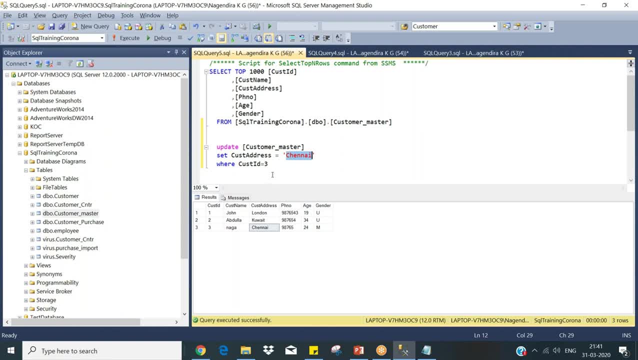 bangalore now you updated to chennai now. now, this is a repeated task. people will keep updating the location, phone number, all those things. so this is the statement i want to uh, execute each time when there is an update. okay, so such a scenario is what i will do. 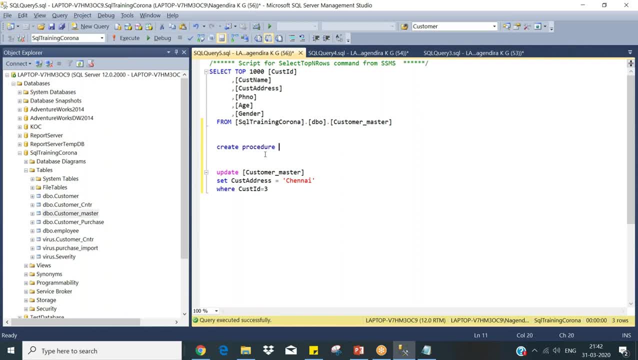 create procedure- customer update- okay, and the procedure, if you can have any without any parameters, also okay. if you keep like this, it doesn't get any information about the customer or what values to update, so you need to create a parameter here at customer id, okay. so remember the symbol. 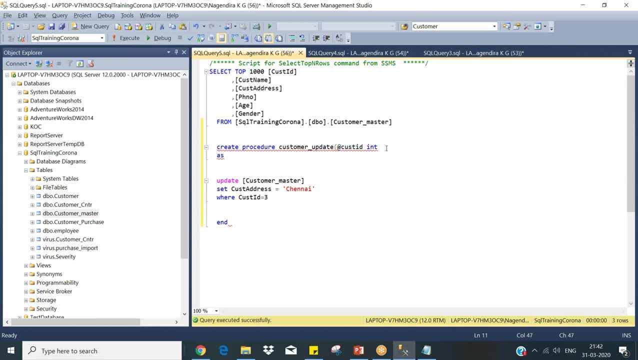 that indicates a viewer variable. okay, at customer id comma at address, you need to define um the data type of. obviously okay, what is the data type of master and worker? keep same as whatever you mentioned: hard file. okay, ette is only the data type. is that where? uh? 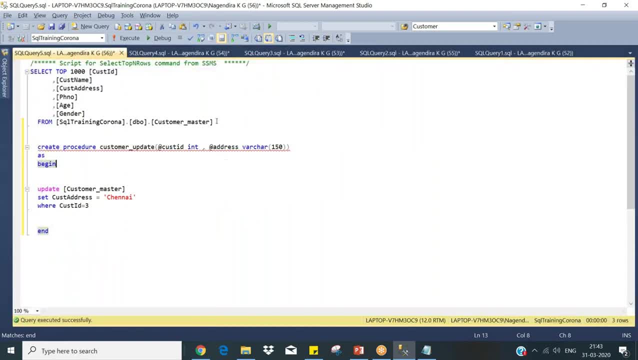 this is the video posted is gonna show: yes, let's check that one. and here 빠�ke Diego. then we go here. okay, so i have just made device name with parameters. okay, so we can start with the vagina, then begin- okay, begin should be the thing, then end, okay, guys. so now i have given these two things now here. then whatever values i am getting it over here should beraine and IT nd, then whatever values i am getting it over here should be pal. 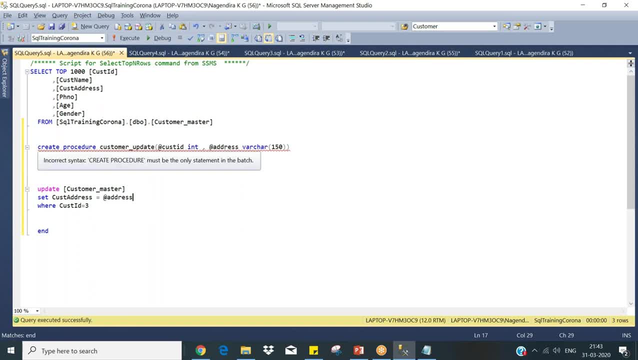 Okay, that is what. replacing the hardcoded value with whatever you pass got it guys. So, yeah, see if I have a hardcoded value here. okay, Let us see. like the main purpose of creating a procedure is like there are number of customers over here. Okay, Maybe I will take. someone has a huge data, six to seven records. Okay, 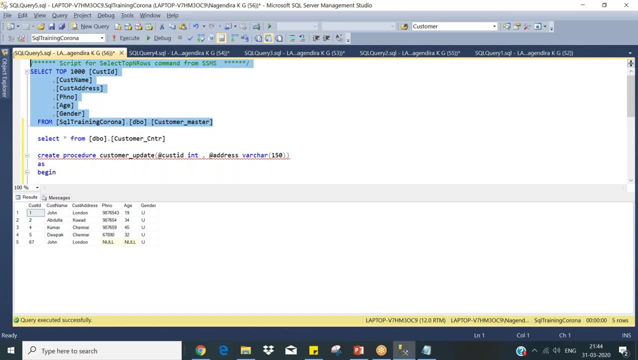 Here you have five records. This is far better. I'll take this, David. See, you assume you have a. we have a customer. You have thousands, of, 10 thousands of customers, Okay, So basically, we want to update phone number customer address frequently. So how you will do it? People enter in the screen. 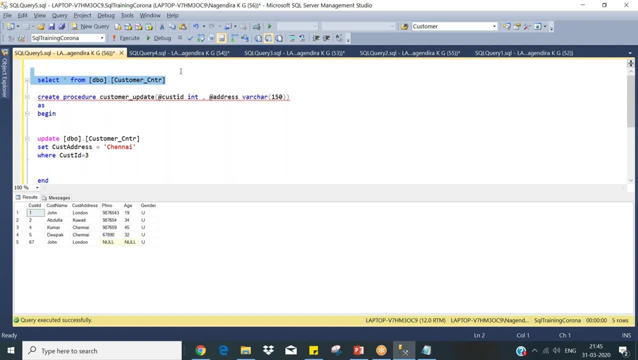 in the GUI front end. then you capture those value. whatever you want to modify, you will capture that value And for you, whom you want to apply for that particular customer. So obviously in a customer table only you want to apply, So you need to get these two. 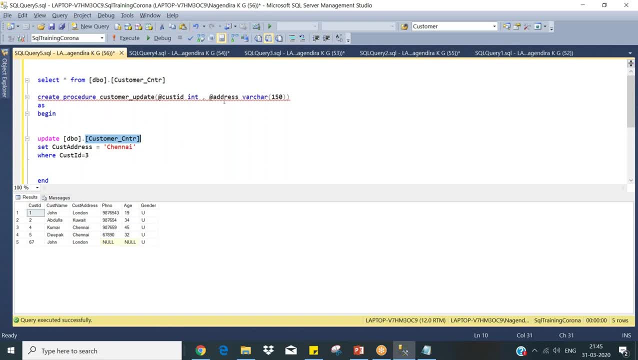 information, what information you need to update. That is for now. it's an address and for whom you want to update. for whom is customer ID? So these two things are very crucial things that you need to capture from the input system. Okay, That will update it. Okay, Based on. 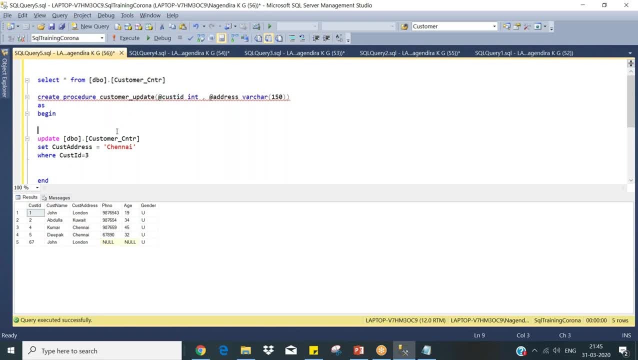 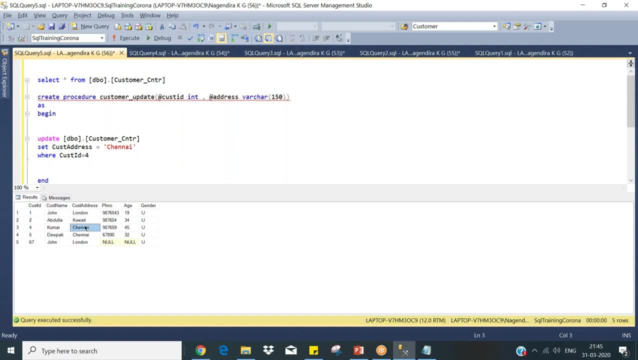 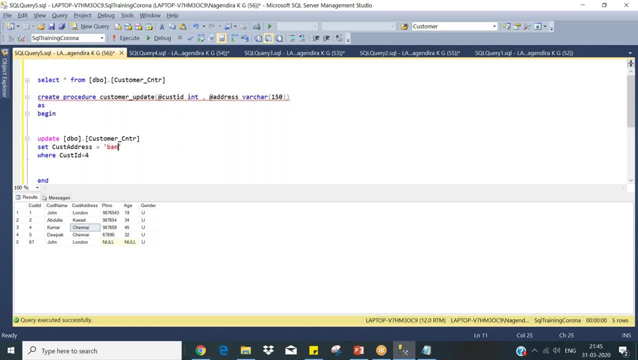 China. When I want to, a he's changed to Bangalore. I need to write Bangalore. So, as you like, you keep on storing this information. what do you want to update, Then? you are not going to update it manually. You should not do it, because you have 10,000 customers. You cannot. 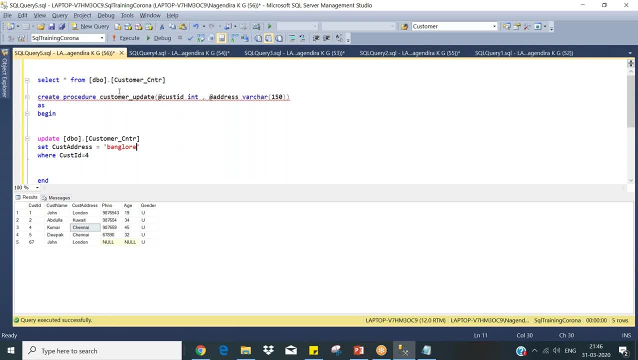 have it one by one. Okay, Instead, what we are doing, we have written a procedure, program, programmatic approach, where you get those information- customer ID and address- and in this place you replace those values instead of for see now, first I will update for Kumar, I will update to Bangalore, so how I can do it. 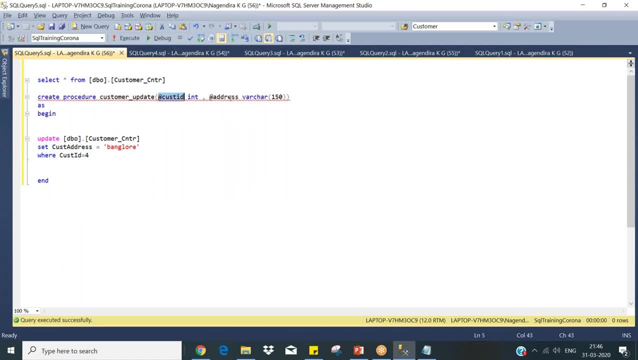 programmatically I will pass for. and Bangalore here. okay, in this customer ID in Bangalore. so this should update me that Bangalore information. now you see he already changed to Bangalore. now I say he moved to Delhi, comon move to Delhi. so I should not make it dynamically, sure, should you have to make? 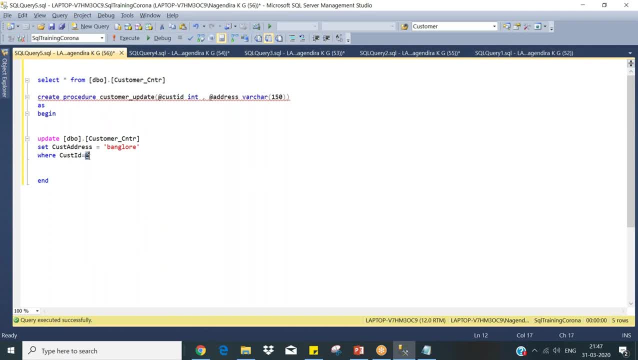 it dynamically for any customer I change. I should not hot code it, so just replace these two values, the hard-coded values, wherever you wish, and whatever values you are getting as input. you put it here. now I create this procedure. okay, now you see the value here now: one, two, three, one, two, four, five, seven. 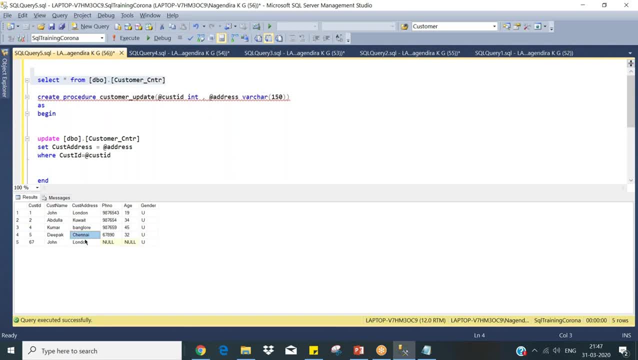 now i want to update deepak from chennai to delhi. i can use this procedure: execute you give a values like you need to give the value five comma deepak. i want to change him to delhi. now i'm not running the update script, i'm running this procedure now. 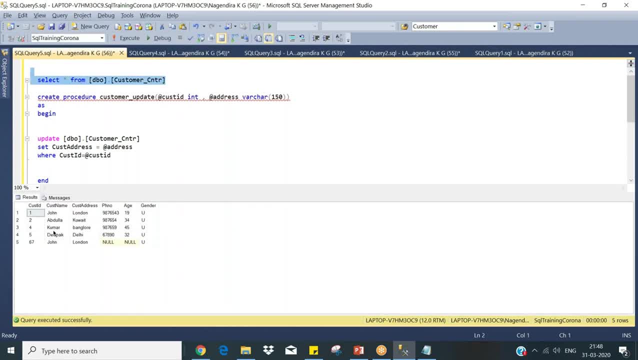 done so. you see, deepak was in chennai. now he got updated to delhi. now you want to do it for abdullah? he's in quiet, i will move him to. abdullah is two. i will move him to somewhere else. i will say africa. 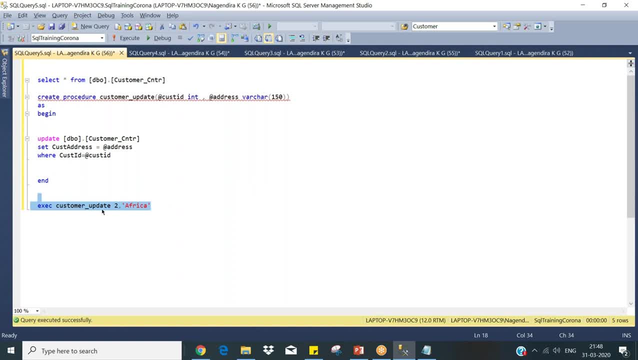 see, guys, abdullah is in quiet. i'm just running deepak right now. so you see, for now we will do it for abdullah. now he got updated to delhi. now you want to do it for abdullah? he is in passing it here, but how it get this is not referring any table, I'm just calling. 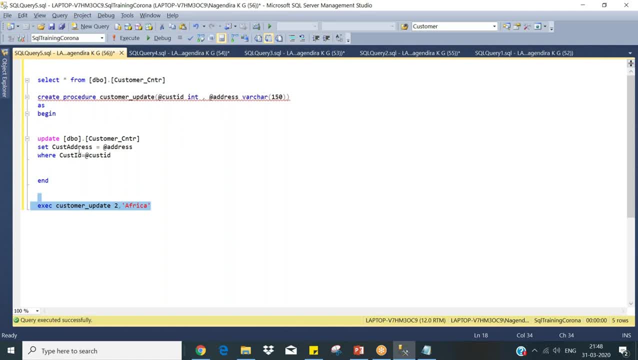 this procedure to Africa, the logic, whatever I've written here, that updates the Abdullah to Africa. you got it guys. yes, many doors. so this is this is how you need to create. this is the main purpose. you go for a procedure, any kind of operations that will perform your 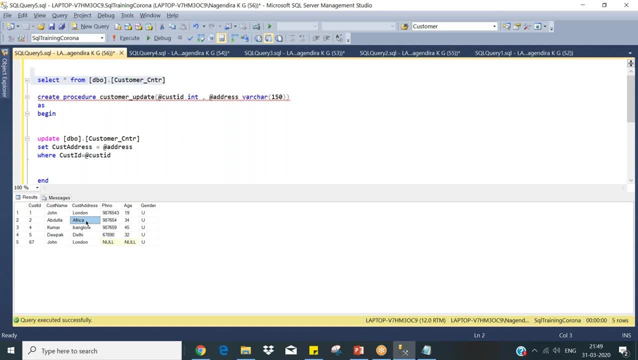 data manipulation: language updates, deletes inserts, regular inserts. so into a table those things, you store it in a procedure. so all applications, your windows forms, web forms, will access to this procedure. they will pass their parameters, like customer ID or customer name, whatever the key attribute that will pass in this parameters, so they will 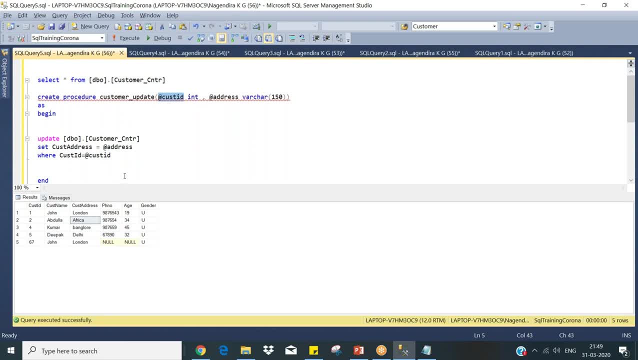 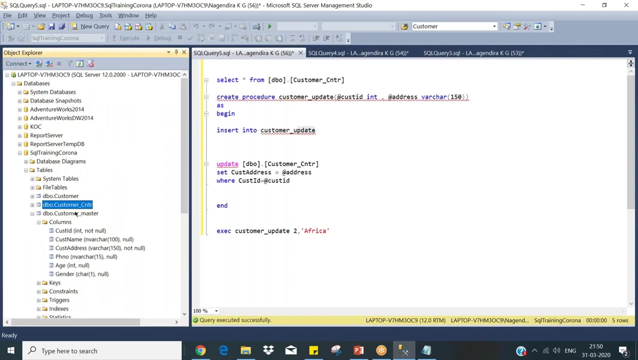 capture it here, then it will be passed here. this is the thing, guys. so you can do any operations here. even I can use the same statement here for logging also, so it is not only one statement in certain to customer master. whoever I'm passing here, I can do a log. so multiple statements you can do, insert into select. 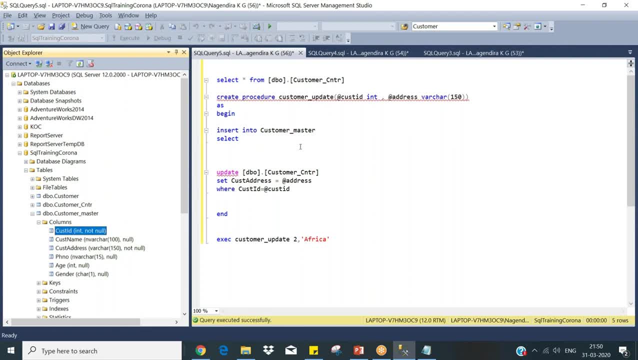 what are the columns? only a name is not there, one is that? no, so I have only this information here. one, I mean customer ID comma address. so how? so now I have created the procedure earlier. now I'm changing some logic inside this. this is the logic change. earlier I had only update, so now 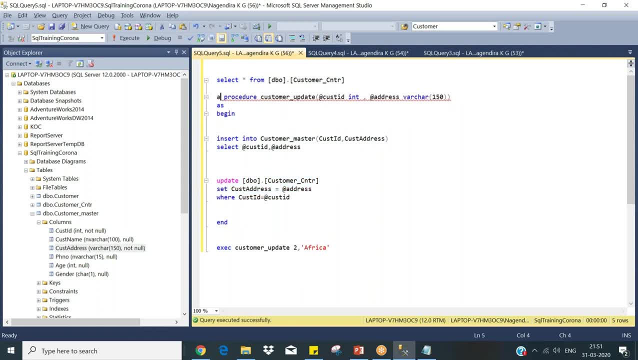 I'm changing little logic, so it's: the command is as usual. you are changing the structure, just create. I mean change the create to alter alter procedure. procedure name: same thing, just use this one now. you see, I have our two tables now. select staff from customer control: customer master. 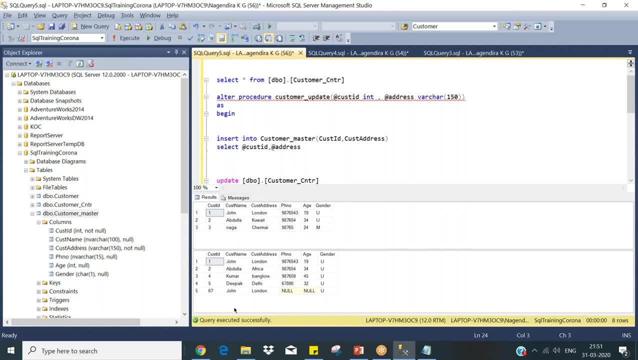 ok, now we are. Now I will say: for John 67, I'm changing him to London to 67.. First I pass 67 to London to UAE. Now what happens earlier? whatever we did changes. there is no entry here. 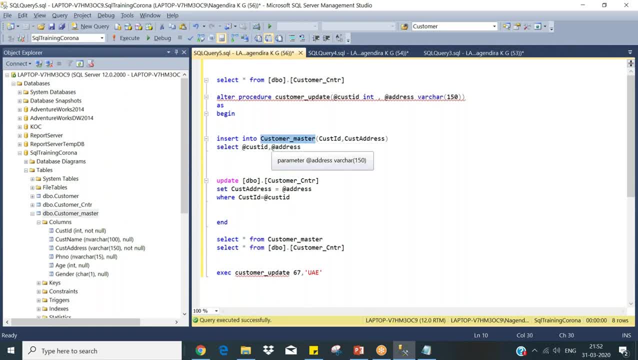 Now I made a logic to insert entry into Customer Master as well. Customer Master: only two columns will be inserted: ID and address. there won't be any names. okay, just for your understanding. It's not a proper way, but still. 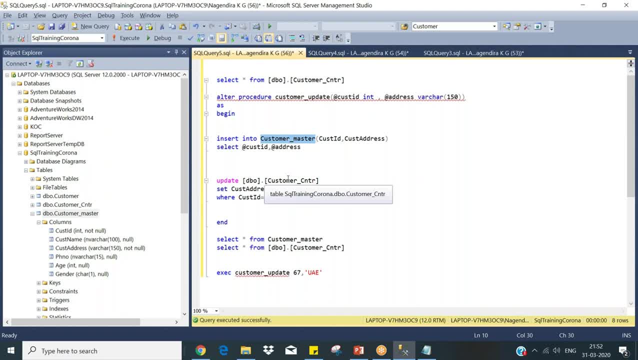 So for 67, UAE will be inserted first, Then for John, UAE will be available here. That is the expected output. Let us execute this. You see one row affected, one row affected Inside. what rows affected? it will be duplicated in your results. 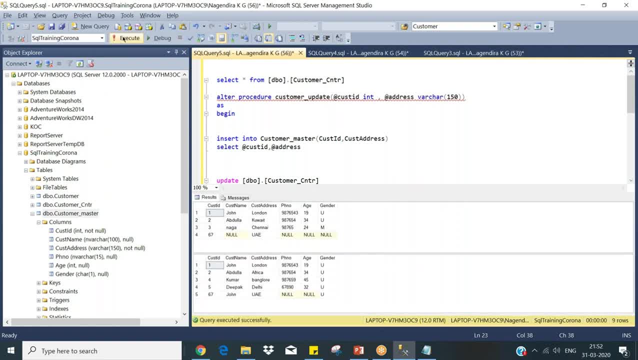 Now I will select the data. So now you see here another entry in Customer Master table 67, UAE. And for John, we have changed to. the address is changed, okay. So this is the thing, guys, about procedure. 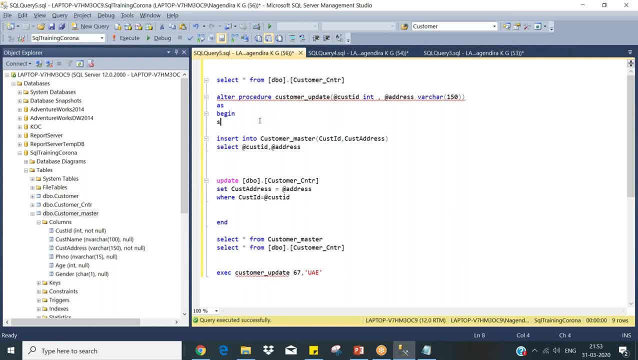 It's very simple as that And something like. we can have a set no count, Set row count on something. Row count on off, set row count. There is some function that will say: like no count or something. This is the. this is useful. like no count off, no count on. 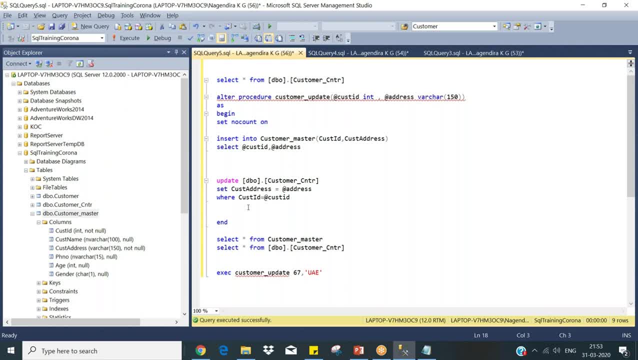 So this is useful when you have. So there is a cast in world when you run this query. I mean earlier, you see like row counts on. I mean one rows affected. one rows affected. message was displaying. 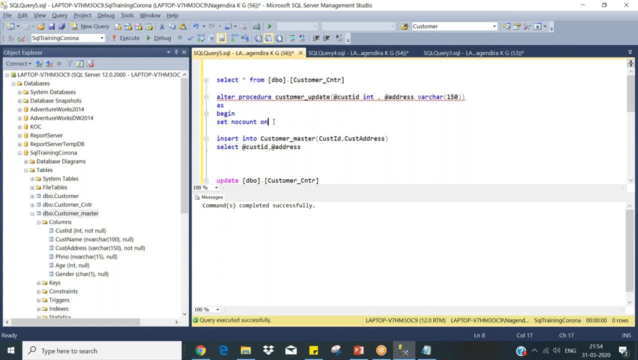 So this itself will take some time. So this is: people say like this is one of the performance improvement factor. So in our- So you have to avoid such messages. you say like set no, count on off something like that. okay, just for your understanding, I'll mention 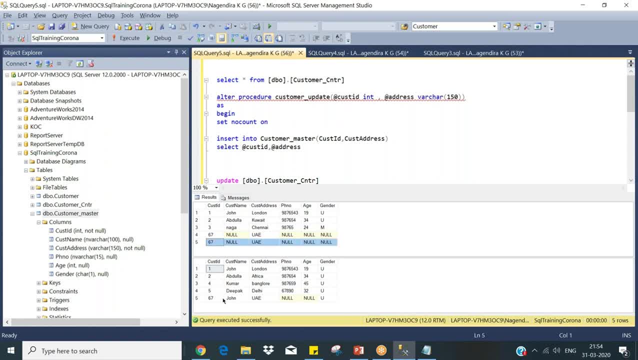 Okay, so when I executed it again, so another entry was there, so there is no changes in your data here. So this is about your procedure, guys. Any doubts on this? Procedures views Go to procedures. Hello. 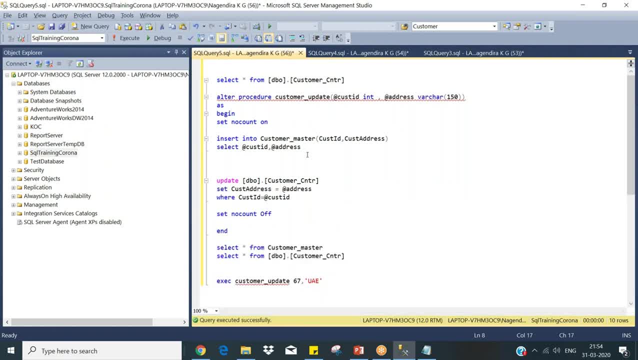 Hello, Hello, Can you explain this again, This technical problem? Yeah, So when I had this one removed, you see, like add that procedure. like this: when I update you, you get a rows affected message. 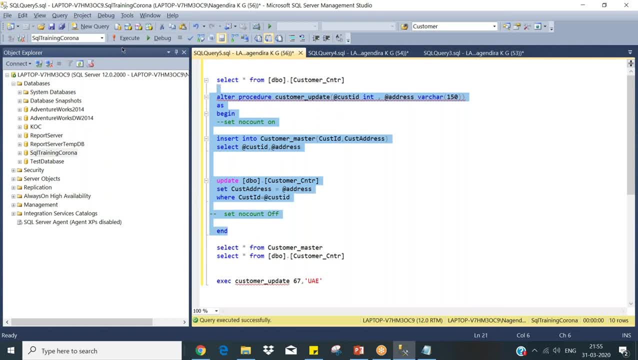 You see, like all that procedure, like this: When I update UaE, You get rows affected message. When I update UaE, You get rows affected message. You get rows affected message. rose affected. rose affected. based on the insert statement. here this message is displayed based. 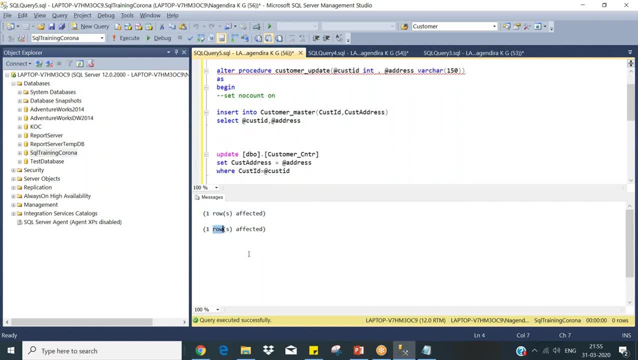 on the update statement. here the second message is displayed. sometimes what happens? to avoid there will be number of statements you have. you keep on executing, so that will have a lot of messages like this. so to avoid these messages to be displayed, you need to enable this option. okay, so i'm altering. 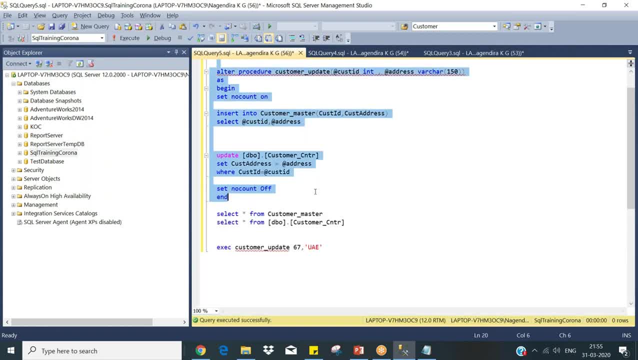 again. now you try to run this guy, omen, i will make him to omen. sorry, sorry, now you. now. you see, like i said, uh, omen, there is no messages now. one rose affected. one rose affected, you got it. it's never. yeah, that is the main purpose, okay. 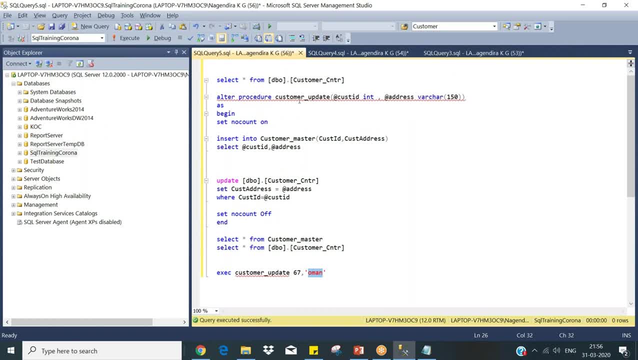 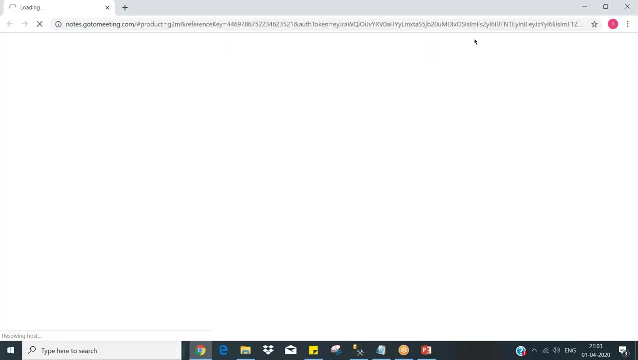 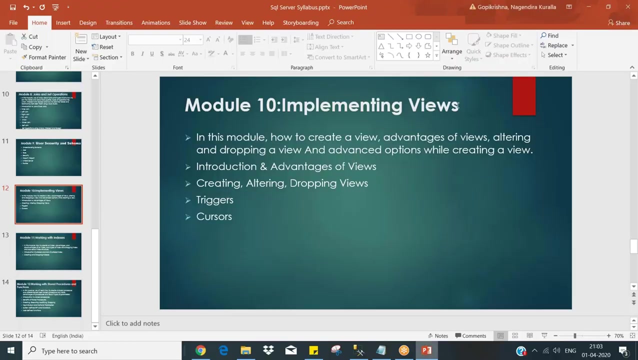 so this is the thing, and similarly, you have one last thing about today's session. we have a procedure, we have something like functions. this conference will now be recorded. so i i read some more points here. it was only abuse and views were there. i will add triggers. 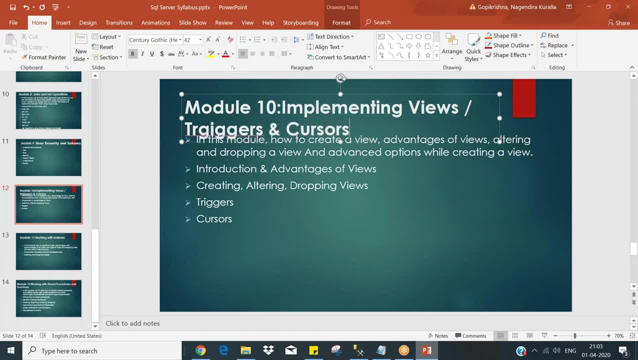 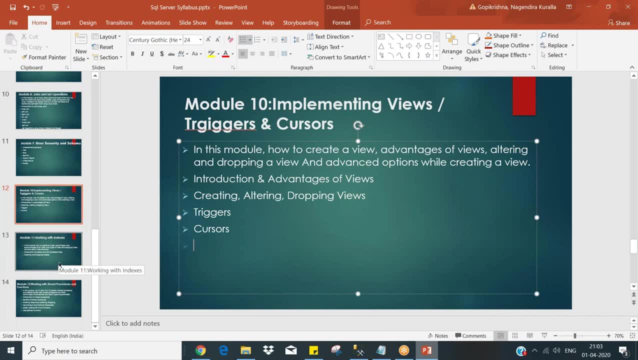 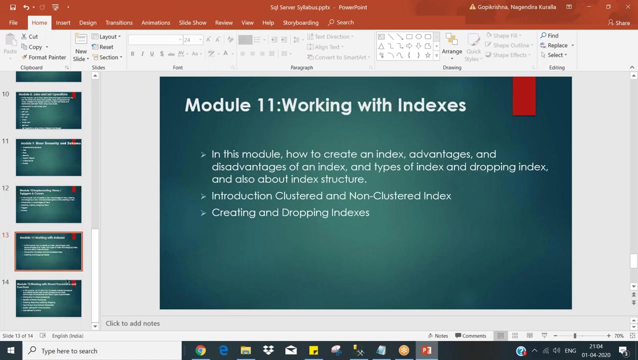 and causes. okay, fine, so i i'm jumping between the topics, i'm not going in this flow. i mean, uh, yesterday we saw about views, then the order over here i need to regram, so forget about that, so we start working on stored procedures and functions. so actually, we saw about short pressures. i will cover some. 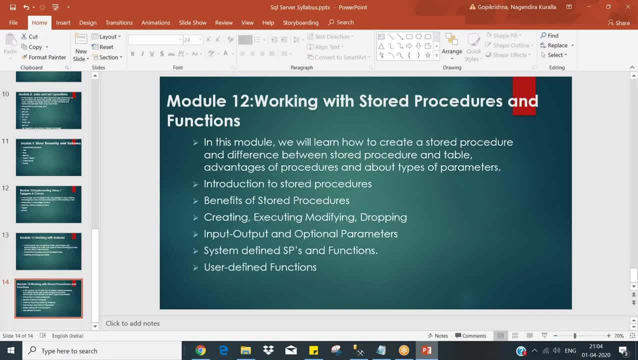 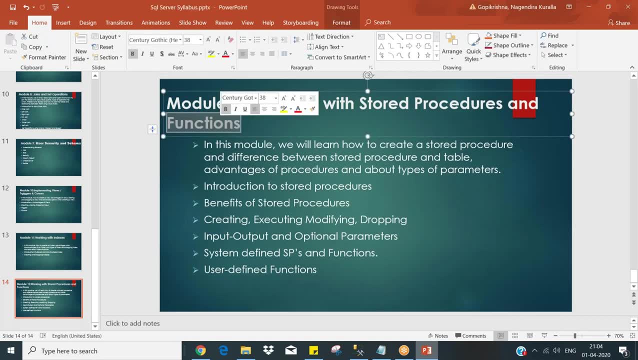 more in that and today we will start. so page three shot at is commission meeting later. bye, bye, bye-bye with the functions. okay, and moreover, what are the difference between functions and stored procedures? that we will see once. i create some function example, then we'll go for it. 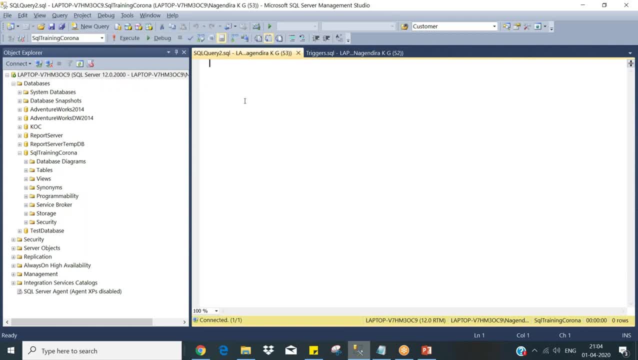 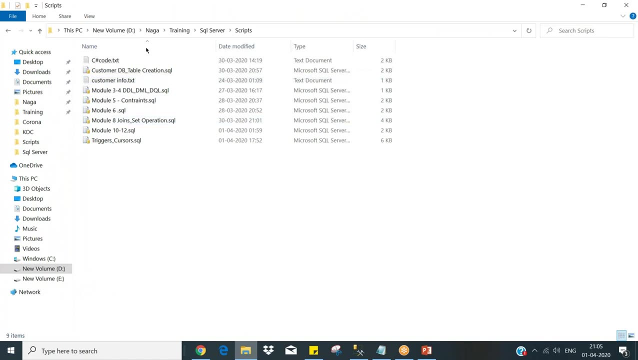 okay, so functions, it is uh again a same kind of thing. yesterday we created a stored procedure and store procedure what it will do, it will do the update. let me check whether i showed that. uh, script triggers, functions, set operations. no, i think i don't have uh that one today. 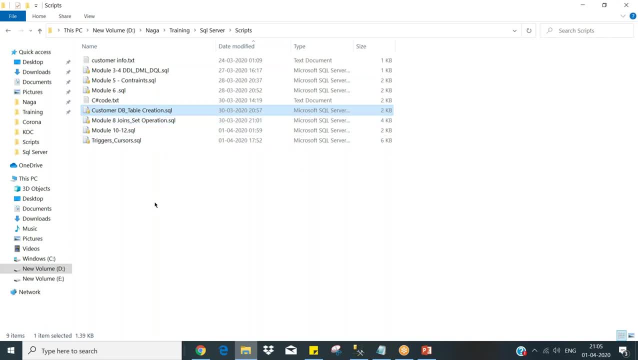 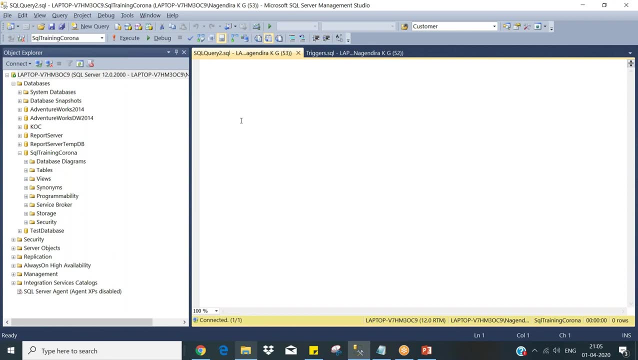 it was 31st of us and some other mode. i didn't say okay. so yesterday we saw about uh store procedure that user to update, that will get uh two parameters. no need to worry, it will be the same thing that we do today. we already have this one here: customer update, so one. 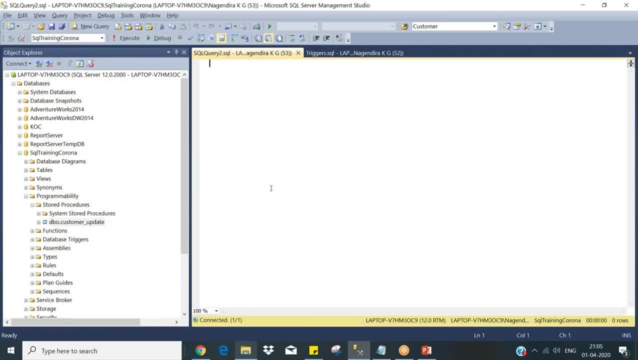 as i said, these are the objects. so your table is your object, your view is our object. you see here, these are the physical structure, it will create it. so tables and we have created views, those things are created as an object here. then you have a store position. this is. 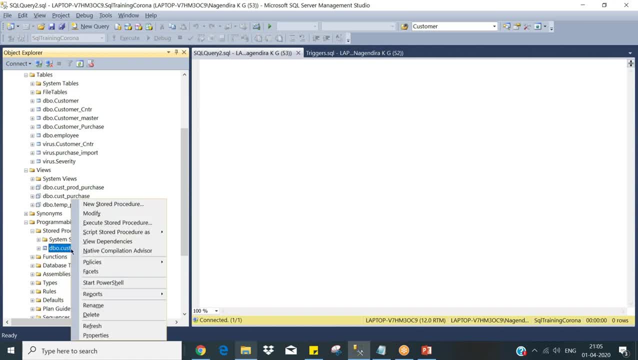 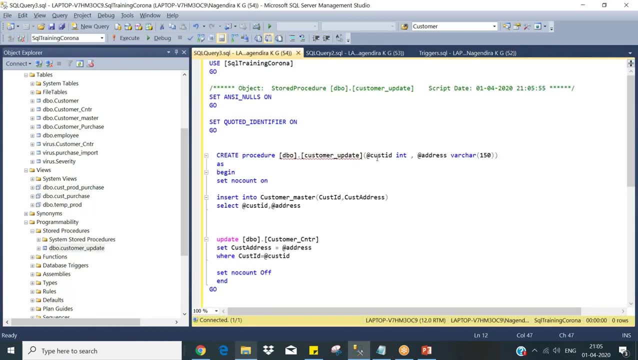 also an object. so these are the things it has created. now you can see the script over here. so what it does, it gives two parameters. one is customer id and address. then it does its job. just it will insert into a table and update the address, both the things it will. 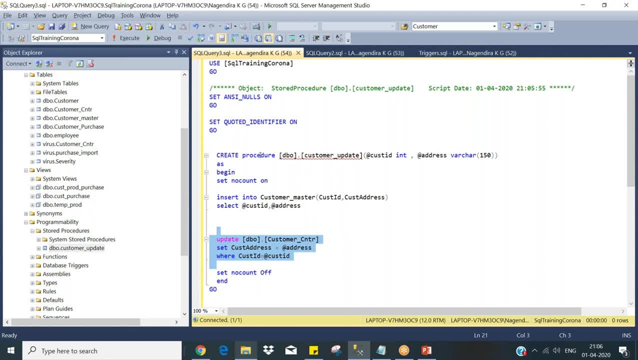 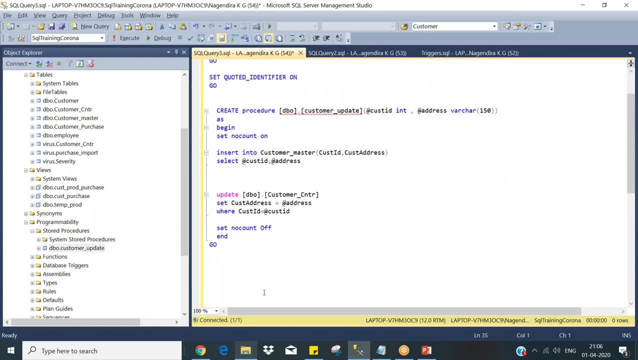 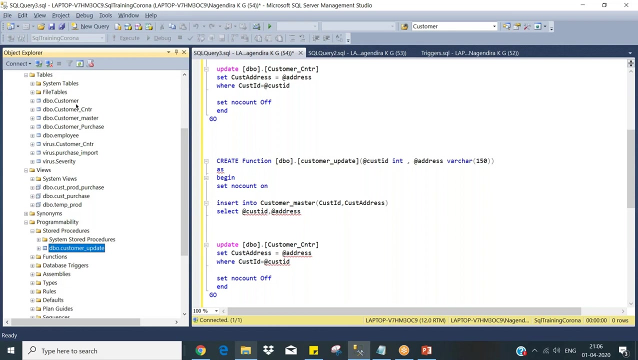 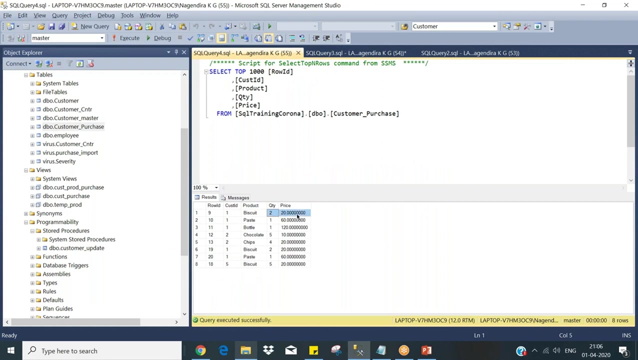 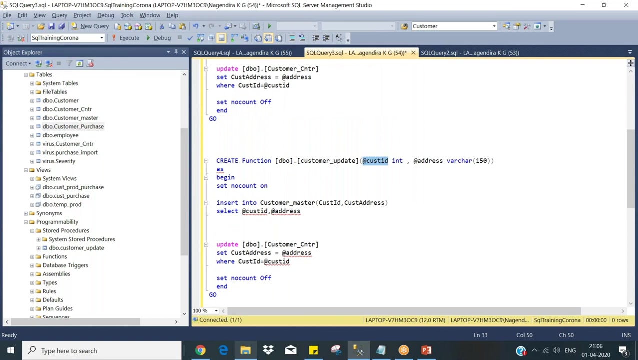 do so like this: operations, if you want to perform, you use procedures, whereas functions, you create function. okay, let me take some table here: customer master, customer purchase, just want to see what it's taking. okay, price into quantity, perfect, okay. so okay, i'll take uh, at quantity, at price. 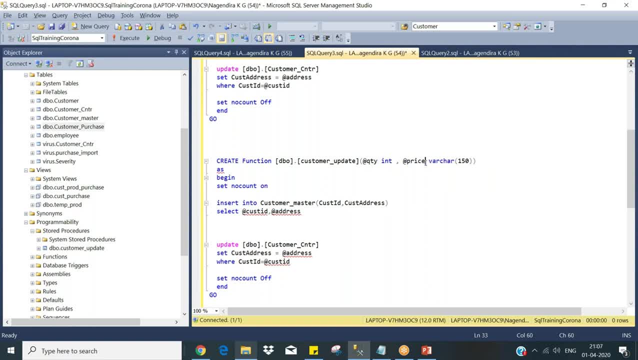 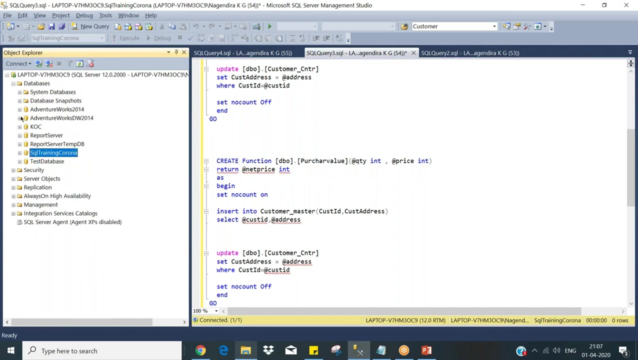 integer again, and this is nothing but purchase value. there is a function name called purchase value and which takes two input, and the syntax is: it should return a value written at net price, something like that. okay, this is the syntax of it. i just found something over here. give me a minute. functions table- valued functions- graph. table valued functions- graph. 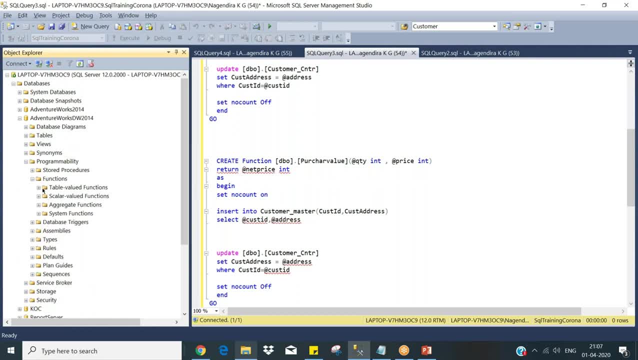 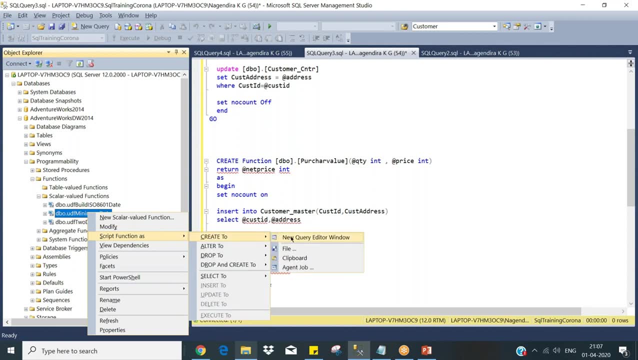 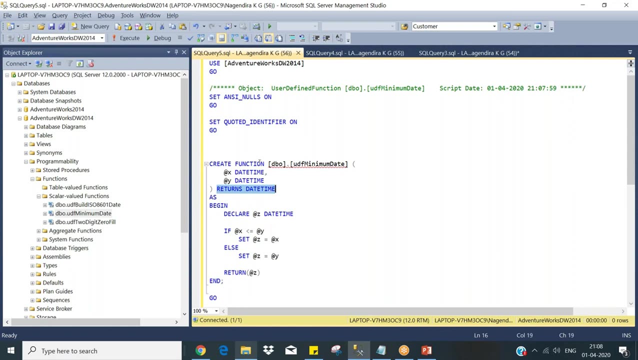 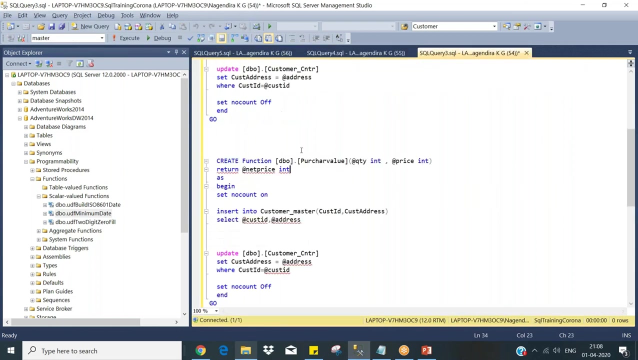 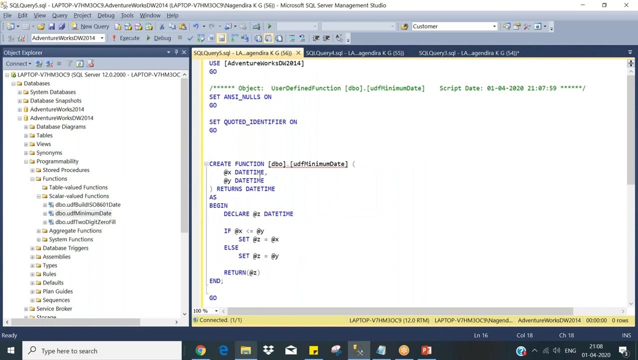 give me a minute. functions- table valued functions. graph table valued functions. graph table valued scale. a valid function- see, basically a function should return a value over here. if you see a create function that will take parameters, that should return a value. okay, returns date, time. maybe we will say return integer. okay as begin. declare: okay, fine. 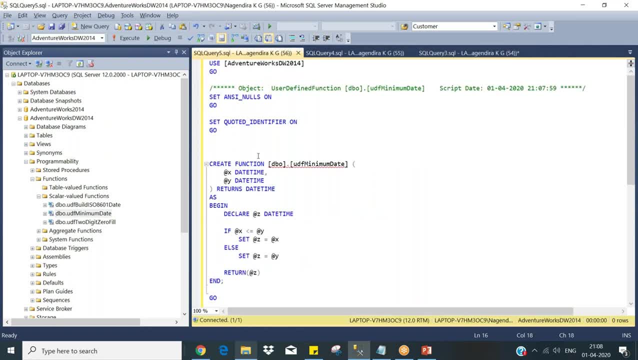 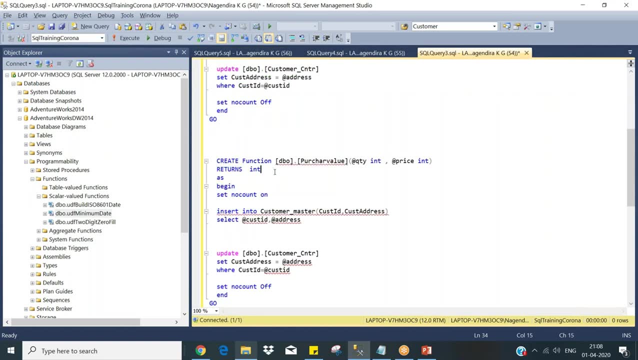 it should say returns. i'll take the syntax from references: returns, integer. okay, that is a problem here. you don't see anything. so what it does is see similar to a programming language. you can declare a variable- i hope everyone familiar with c or what basic languages you can declare a variable. 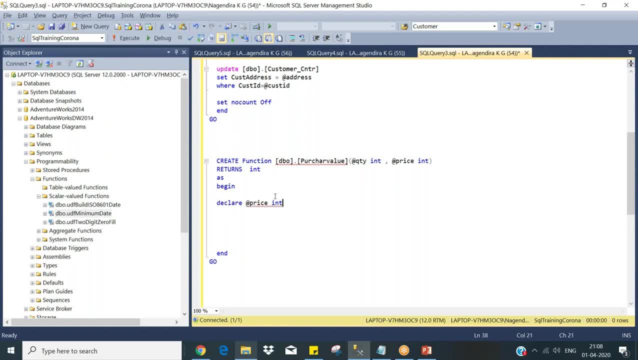 price, okay, and declare it as integer, then what you can do is set. you need to. if you want to assign value to this variable. you can say like: set okay, set price equal to quantity into, i will say net price, quantity into price. this is as simple as that. okay, then what it will. 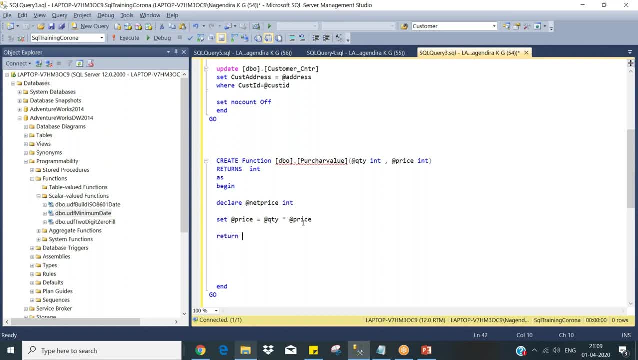 add to do once it calculates, just return me the value, return net price. this is simple programming. okay, that you understand this one. it gets two input variable once: quantity and price. it will multiply and return the results. if you give two and three here, it will return six. so this is what you return: a program i hope everyone has. 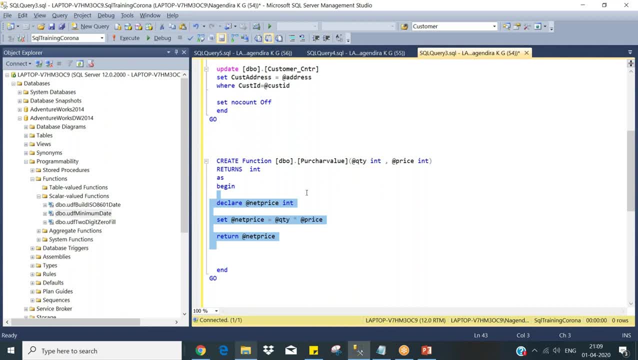 written some programs. if not, this is the way you have to write, so you need to store these results in some place. that is the variable i have created here. this is the way to create your variable. declare is a statement to create a variable that will hold temporary results. so i'm setting the value. i mean the. 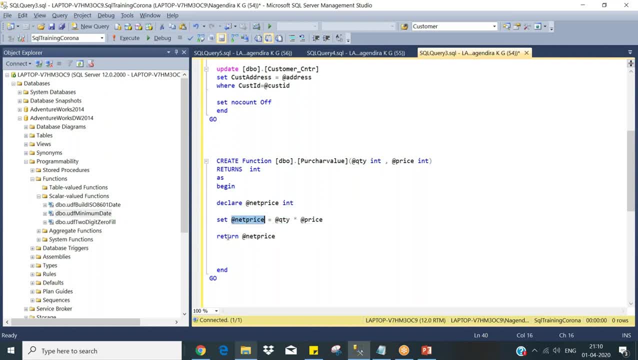 calculation of this will be stored in net price and i'm returning this value over here. okay, this is the definition of your function. then i will just execute it. okay then, how to call them? so i can use select of purchase value and i need to specify two comma, something like that. so i hope everyone knows the multiplication. 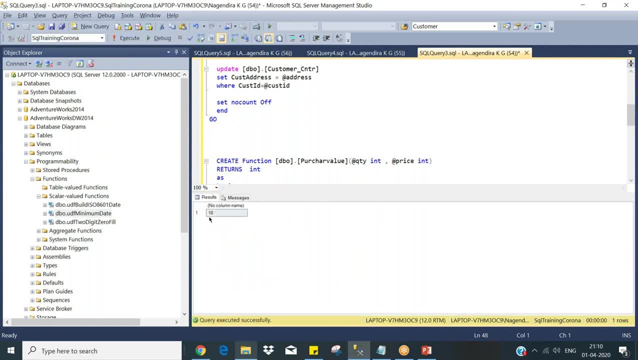 just i will execute: two into nine is 18. i'm getting this value okay. so what is the main difference? over here is like: so you, you guys, understand right these kind of calculations you will create, okay, and you can use this function to compute some values. it is as simple as that. you just imagine. 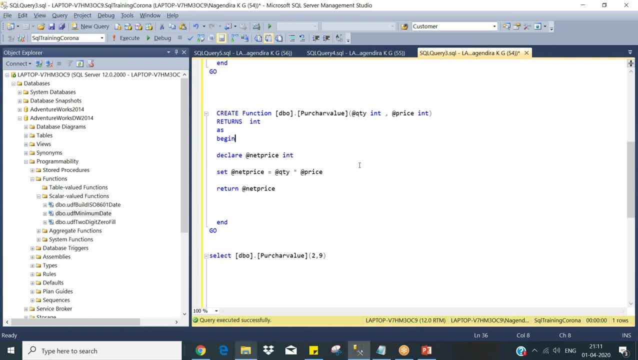 you are finding the uh tan theta- i mean some average values- or you are passing some calculations. like you are passing some calculations, like you are passing some calculations like uh, average for that month, any calculations you can do over here. okay, you pass that value, two input values, then you can execute. you can pass those two values here, then you get the results over here. 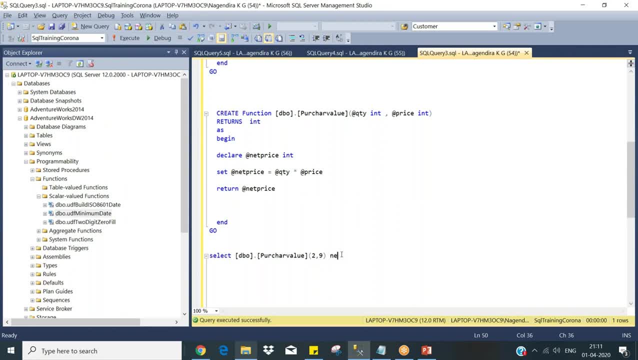 okay, this is your function: net price. i think even you can execute like. you cannot execute a function like this. let me check that one. okay, so you cannot execute a function. okay, you can select a function like this only. okay, so that is the main difference between your uh store procedure and functions. what i'm trying to say is: 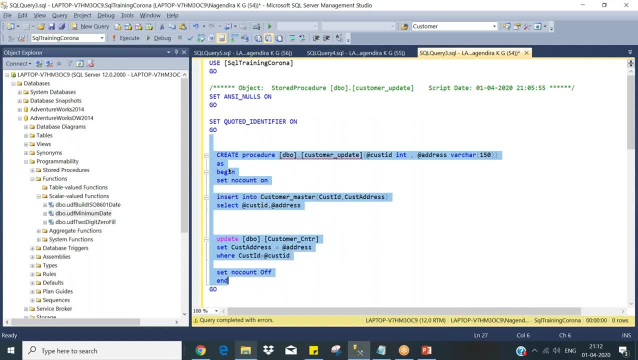 you have here a create procedure over here. okay, create procedure, procedure name. and in order to do a call to this procedure, you use execute procedure name. you pass some id three comma, some bangalore or chennai, whatever, like this: you will pass, you will, you are executing. 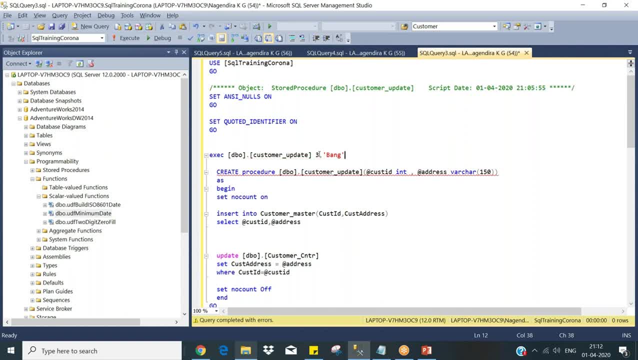 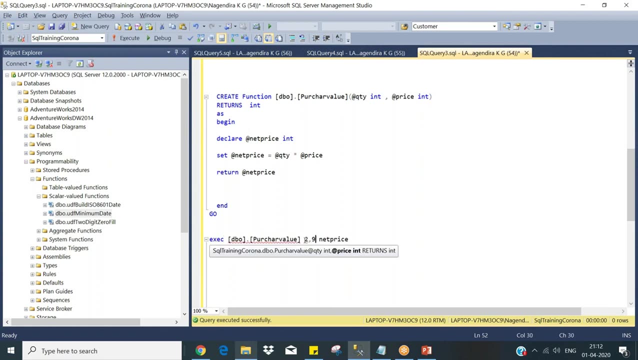 without parameter, i think without parameter, i think you will be able to execute the result. now you got the value. similarly, here, i think you can do it. let me check that one execute will not work here. this is executing, but you are not getting the result. in order to get the result, you need to put it like this: select. 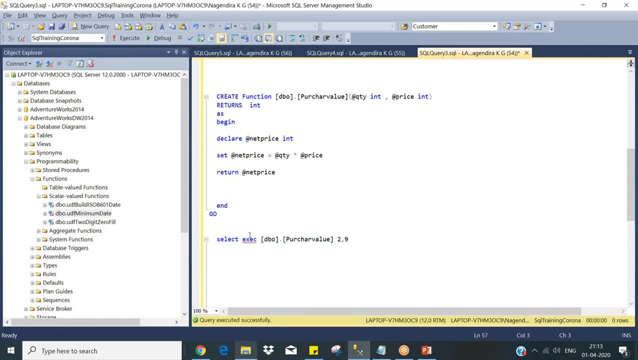 you, you no need to use the select. if you use select, then this is enough. you can get that value in the select statement. i'll use make it click in there, both the guys together. so in order to get the values, you need to use select statement to run the query. now this is the value. i'm passing it over here, 2 comma 9.. what happens? 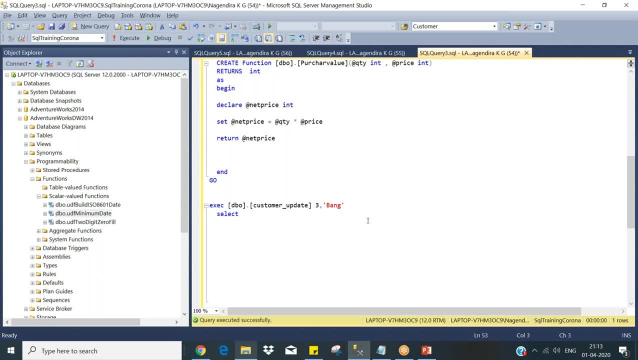 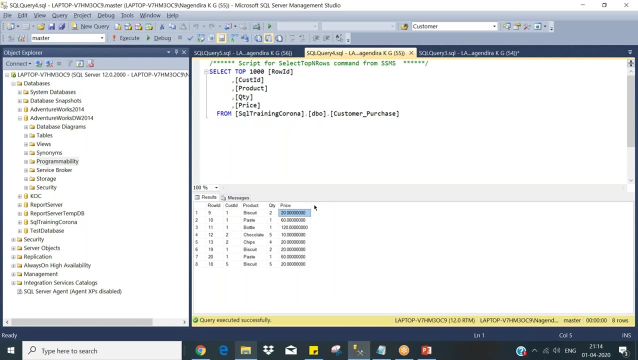 if i run this function for a table, you can do that by passing a this function. so here i found one data: this table. i want to multiply this quantity into price. i want the result 40 to be displayed in a new column. this i want to do programmatically. i don't want to write the code. 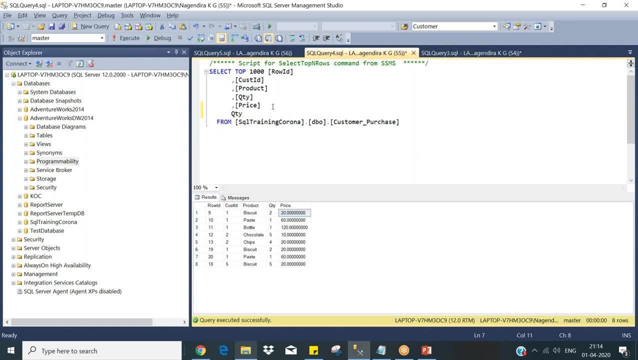 even i can write like this the same thing: quantity into price. okay, this i can do it here itself. i'll get the results. i got this result: 40, 60, something like that. instead of that in this place i can call that function passing quantity, comma, price. that will calculate this: 40, 60, 70.. let us 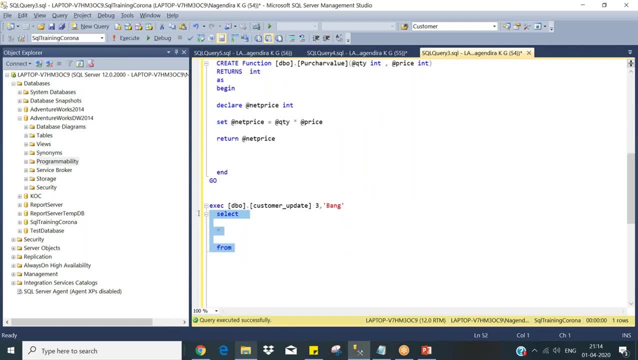 show. let me show that one what i'm trying to say. so this is a table and i'm having the result function. so function. then i'm using this function. i'm calling this function. okay, here you see, in the select statement, i'm calling this function. this is the function. 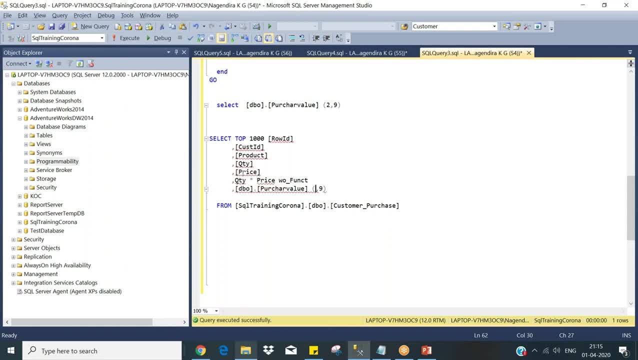 name purchase value instead of 2 comma 9. i need to pass this quantity here, this price over here. so 2 comma 9 gave me 18, so this one and this one should return me the same using function. so this is without function. this is using a function. both return me a same. 5 into 10 is 50. 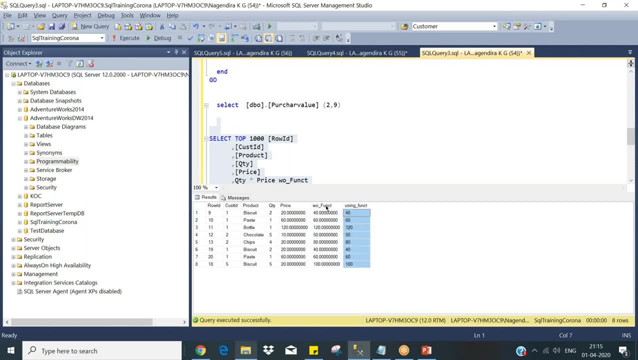 5 into 10, 50.. so using a function, this returns. this is without a function in the direct column, so i have written it like this, because some calculations you cannot do it in a simple calculation like this. okay, some calculations. you will pass these two values and in your logic. 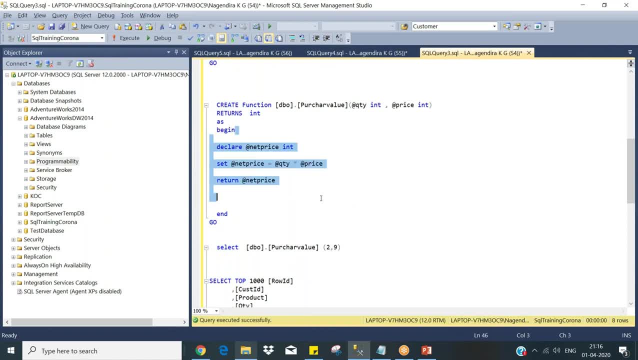 you compute lot of things over here, you write hundreds of codes over here. then final results should be passed to this column based on the two input values. so such a things. you go for function and the main difference. now you got about what is the function used for and the stored procedure also you can do. 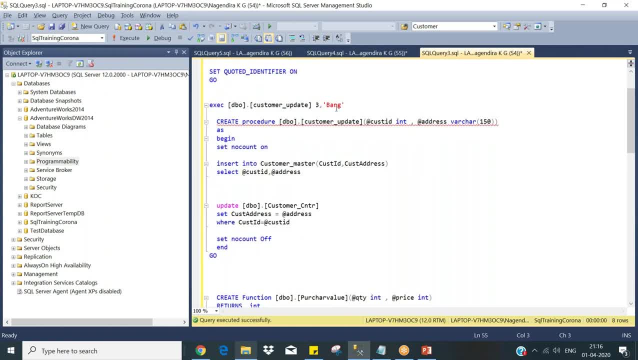 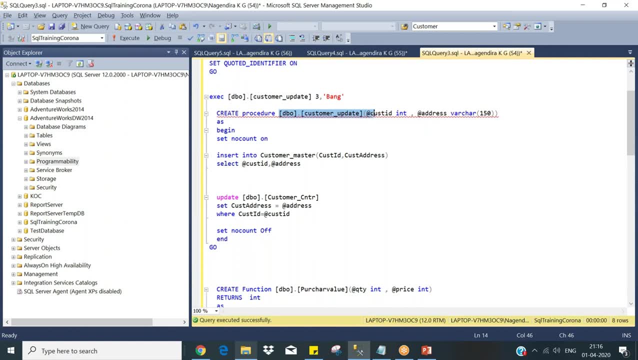 it the same way, but you cannot use it in the select statement. the stored procedure, you cannot use it in the select statement, say for example: what i'm trying to say is: so, since i said, like i can pass parameters here, so this customer id and address also i can pass. right, you might have asked. 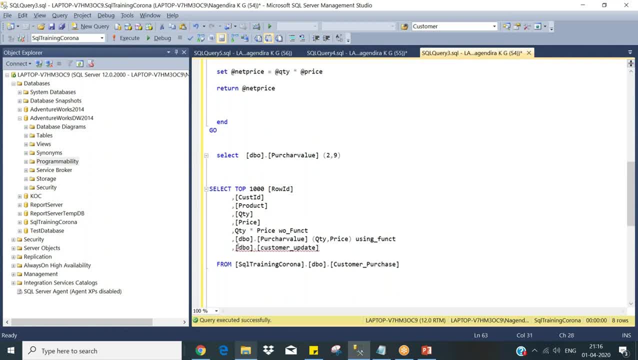 so this is the stored procedure. customer update. since the stored procedure requires execute statement explicitly mentioned. okay, you cannot have a select statement and the execute statement over here, so you cannot use a stored procedure in your, uh, select statement. okay, that is the thing, but whereas you can, 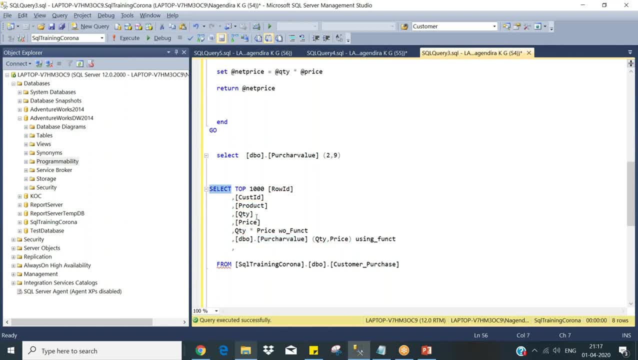 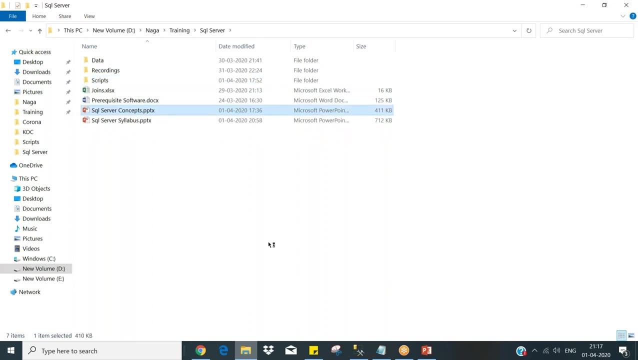 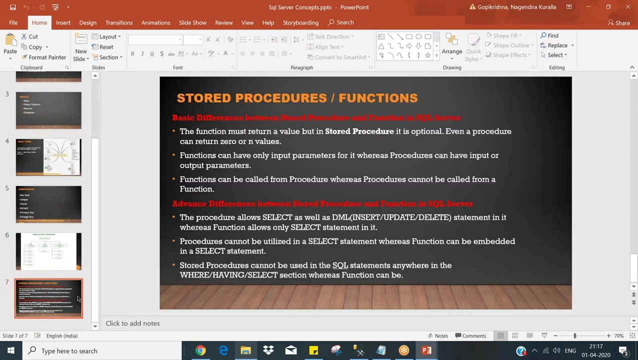 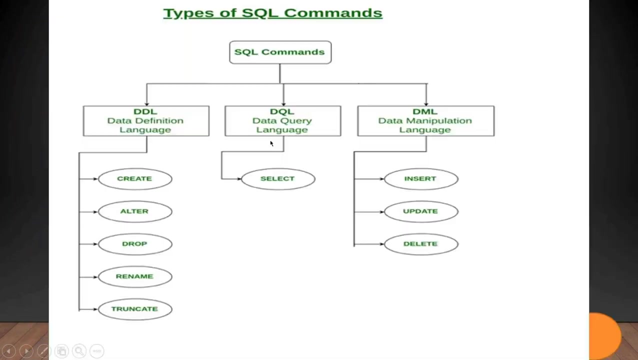 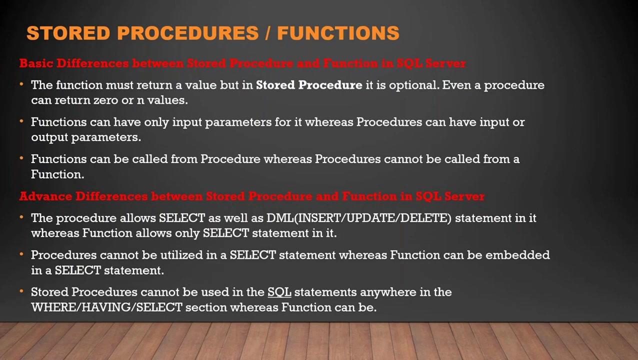 have your function in your search statement that will execute for each row. i hope i am clear with this. let me show you uh base difference between these two. so stored procedures and functions are the same. so you pass standards when you have any setting, even now on the second page. 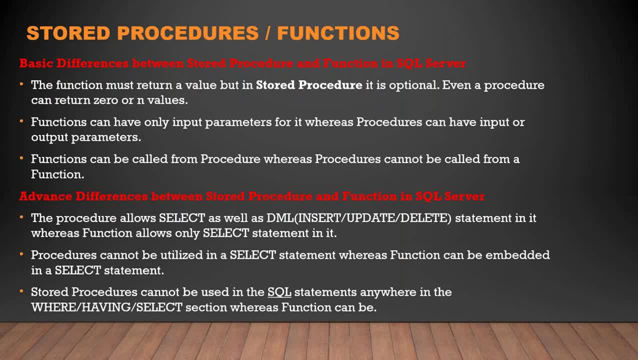 or in the second class of your Mittens. do you want to forget to put any button? but actually you do it like that by pushing alt. right, then it gives you some hören. see here, modified it now again. see it: this change as well and you see the most. 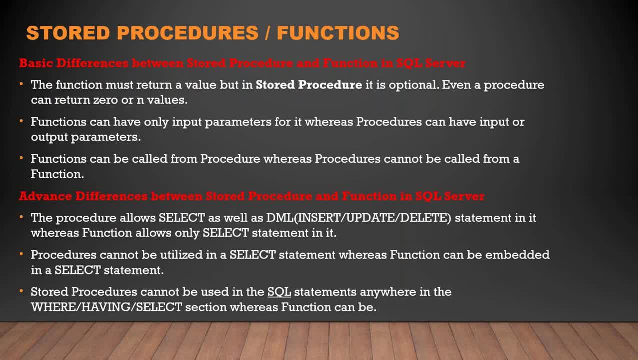 important things. that comes one. the first is the insta change. it means it needs to be removed or before installing. if it is not installed, inflate it. this does not workít. Gobierno, both do the same thing and you show it. whereas that function. you gave these two inputs, it returned. 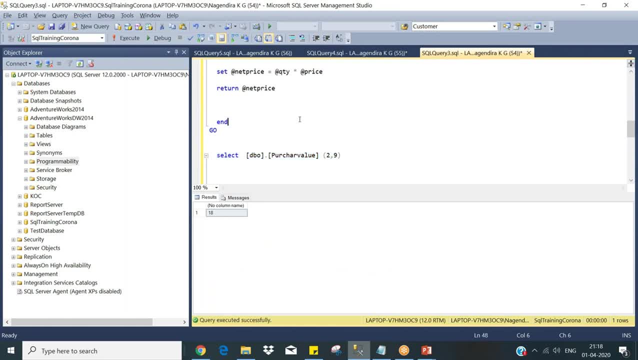 you a value called 18 when you execute this procedure. that does not return any value. this does not return any value, just it has it has done is operation. whatever you do, okay. if you want some operations to return some value, by default you go for function. okay, then store procedure can also return a value. it is not. 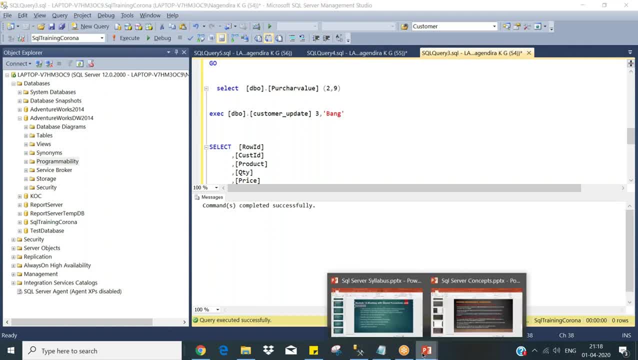 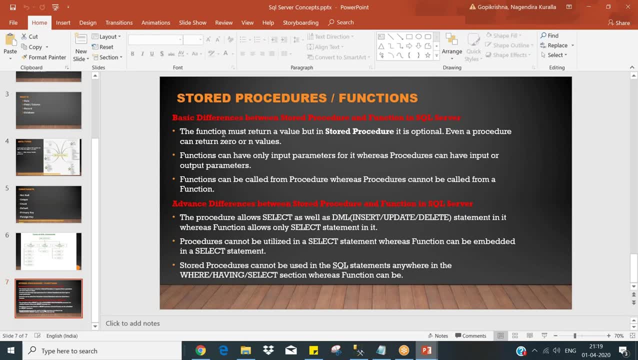 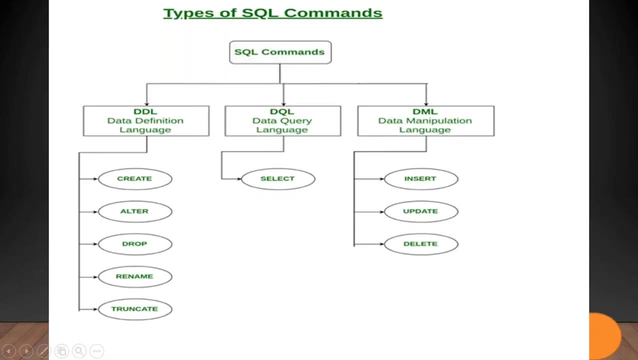 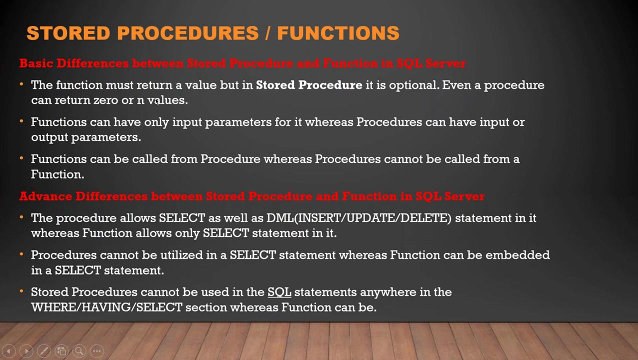 mandatory, like it should not return it's. they said like it's an optional, okay, but short pressure. it is an optional, but when you want something to be returned, then you go for a function. okay. so that is what they mentioned, even as procedures- stored procedure can return zero or n values. there is any? 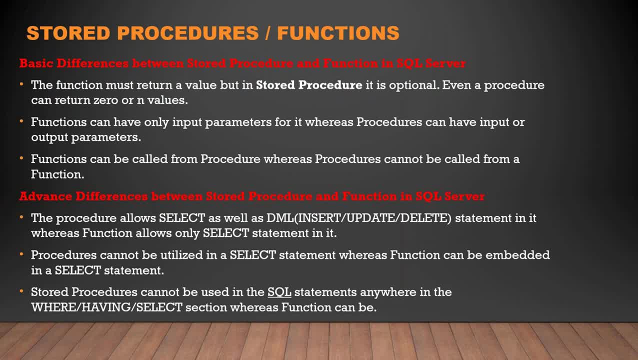 that can return values. that is a code difference. okay, next point is: function can have only input parameters for its, whereas approaches can have input or output parameters. so it is same. I mean more or less so: function should have input parameters, can have only input parameters. only input parameters means: 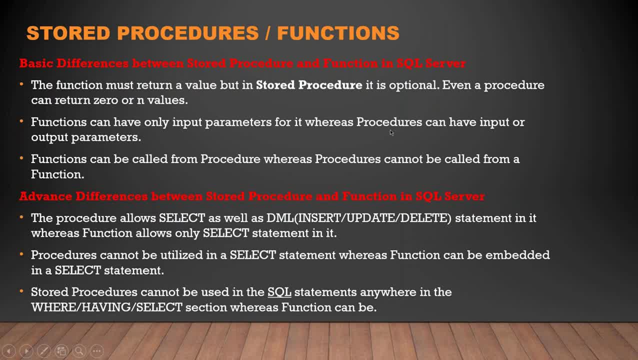 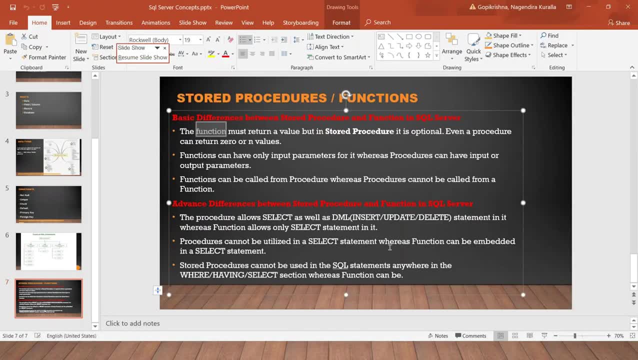 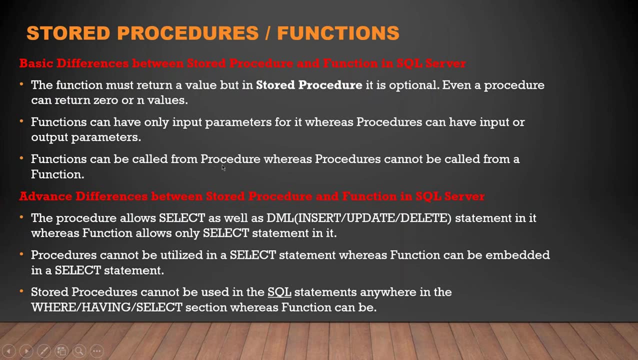 I, whatever you pass, and procedures instead of written value. they say it has output parameters. okay, the parameters matters. whatever you pass here, you can specify. i will tell you later. functions can be called from a procedure, whereas approaches cannot be called from a function. so it's like: uh, some people will have a comment from here to the. 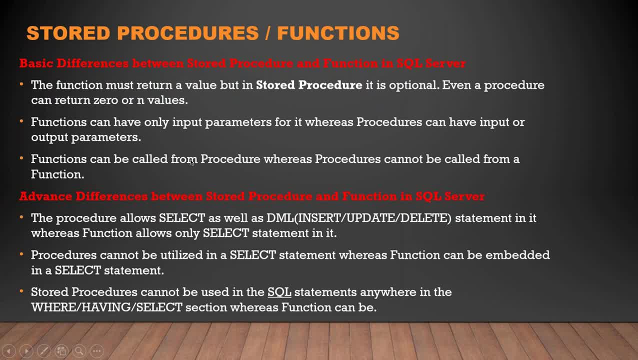 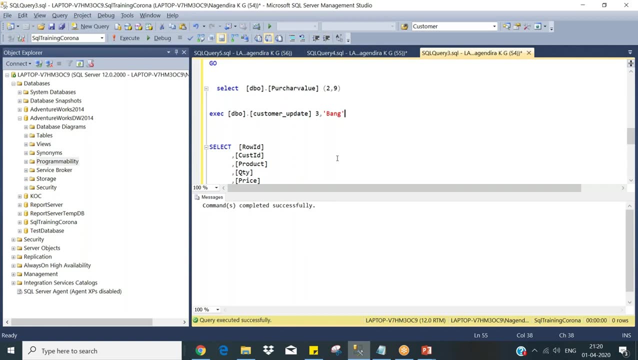 there to the. it is not possible. vice versa is not possible, meaning like inside a procedure: okay, inside a procedure you can call the function, but from a function you cannot call a procedure. that is what it mentioned. let us have that one, these two points clarified. i'm just altering this. 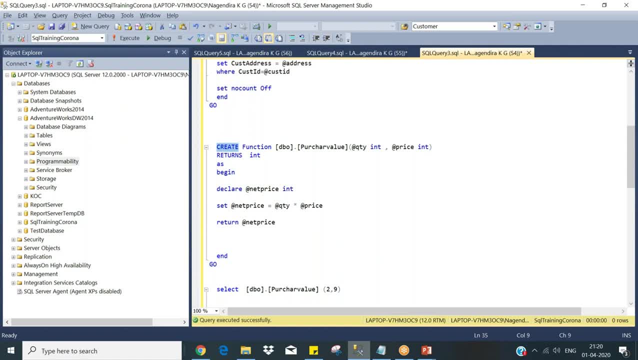 procedure: create function function name: i'm saying alter. so as usual, guys, this d ddl operation applicables. alter means you are modifying something. what they're saying is: i have this function. if i say like i want to call something inside this function, i'm calling this procedure okay. 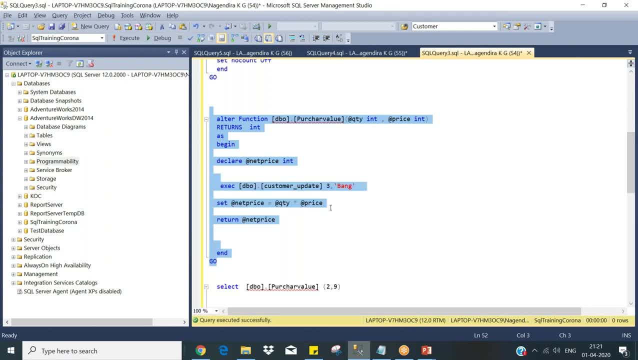 you execute it. okay, now it see it has compiled. compiled means this code is saved, but when you run this one and when you run the other one, another one, it would not apply as well. okay, so if you just, you just execute it from the initial function. so it says like only functions. 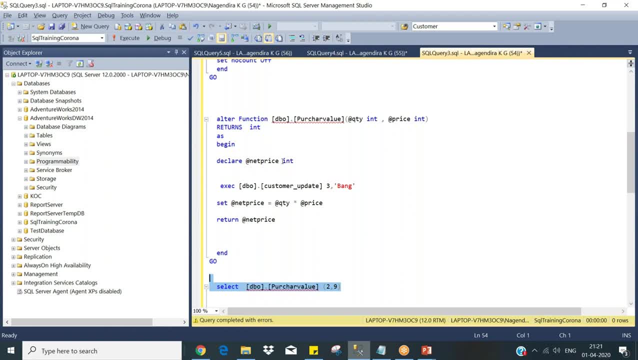 can be executed, another function you can call. you cannot call a stored procedure inside your function. okay, in such a cases you should avoid it. basically, guys, people will confuse where which one i want to use. i want to use function or store procedure when you want to call us another stored procedure. 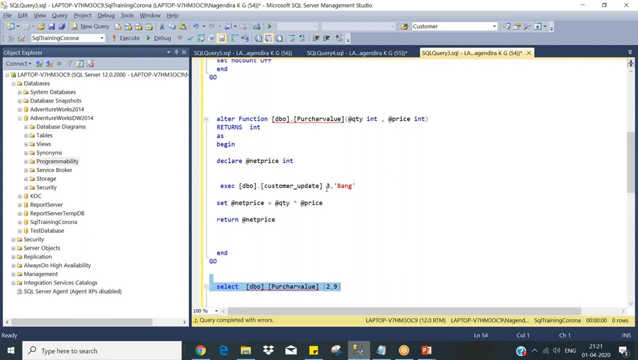 then you go for stored procedure. so stored procedure can call another stored procedure, fine. but you want to do some simple calculations, such a kind of things, or any other complex calculation that returns a value- single value or multi-value, whatever. then you go for functions. this is the simplest way to understand about functions and stored procedures. 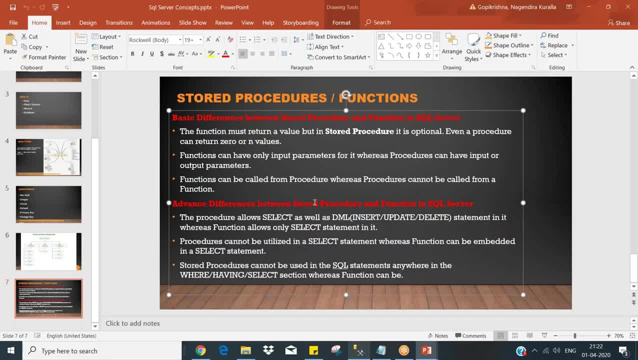 and the other things are there. procedures allows the stored procedure. see, people always say procedures in sql world. they will not say with the short procedure it's procedure procedure allows dml insert, update, delete, whereas function allows only select statement. okay, these are the things you need to consider, what to choose, whether you go for short procedure or function.